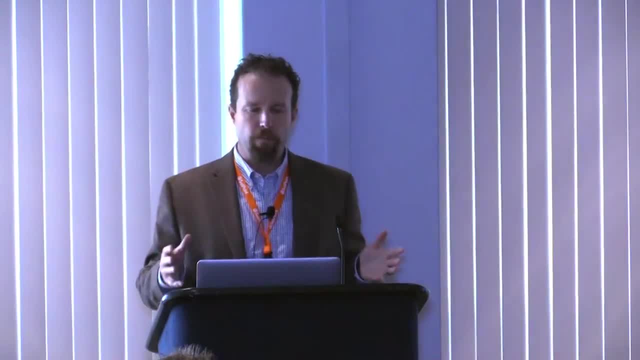 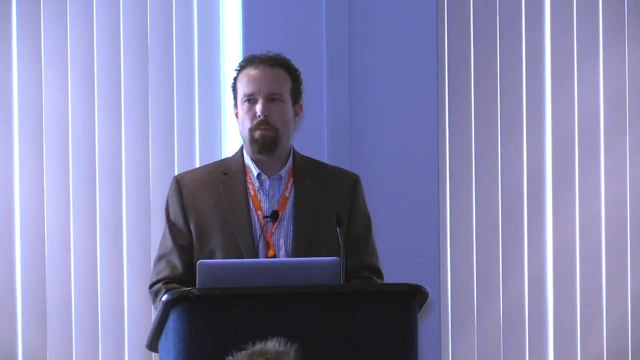 And a little bit of background before we get started. I am going to move fairly quickly through a lot of slides here, But the idea for this presentation really came from the realization I had that we were seeing more and more advanced attacks coming from adversaries against our customers. 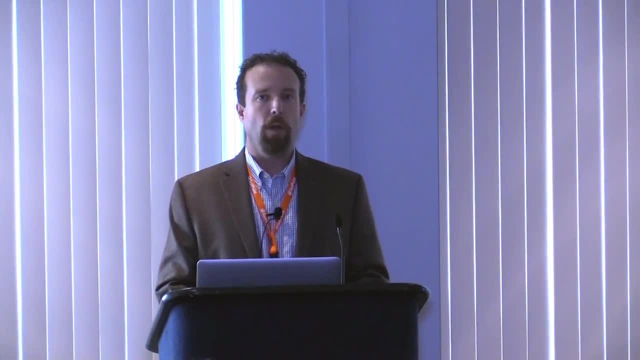 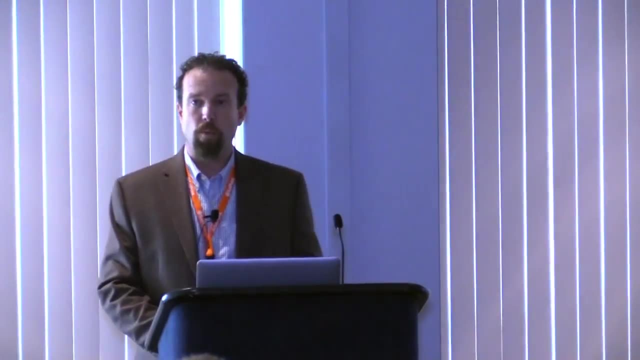 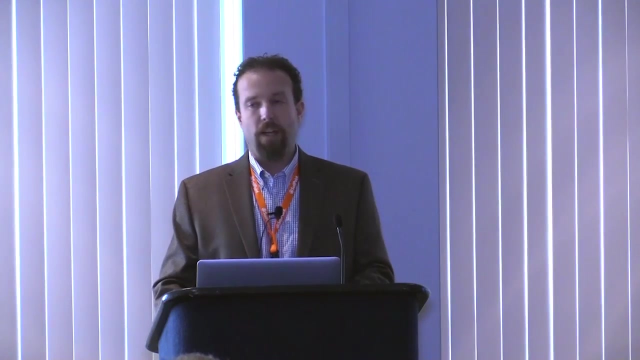 I work for Akamai Technologies and we deliver and secure web applications for global customers. We see anywhere from 15 to 30% of the world's web traffic, So we have a very good vantage point And the realization I had, and many others were having within teams I work with, were that with these advanced attacks, 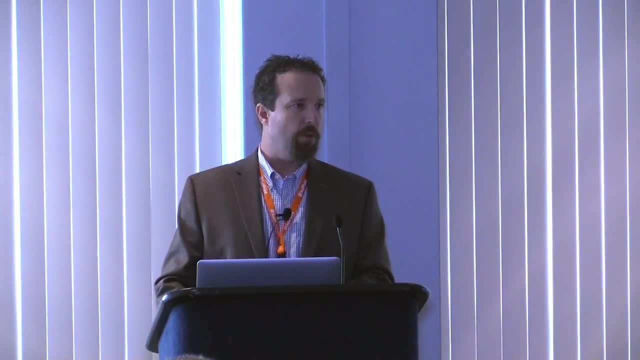 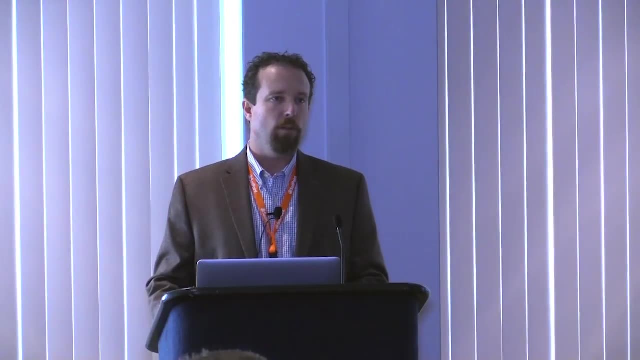 we were seeing the most success with a variety of tools at our disposal, And those tools gave us the visibility and the response capabilities that we needed to really deal with some of these more advanced adversaries some of our customers were seeing. We'll dig into and look at a couple of examples. 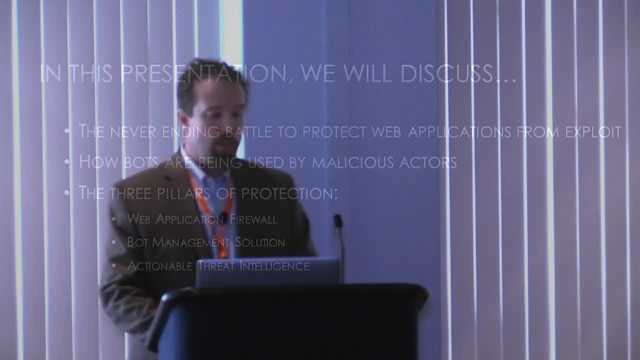 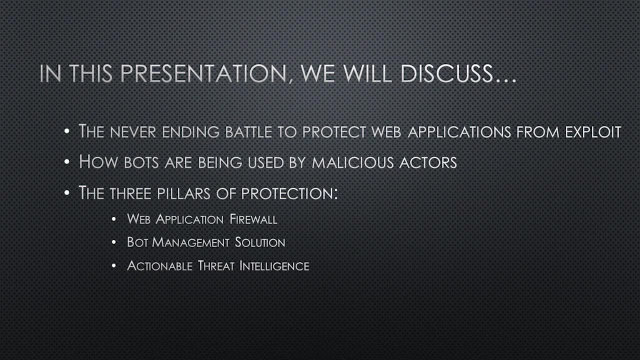 We'll talk about what I'm talking about, But first of all, in this presentation, what we're going to cover. first, take a look at and examine the never-ending battle of protecting our web applications against the attackers that want our data, that want to gain a foothold within our resources. 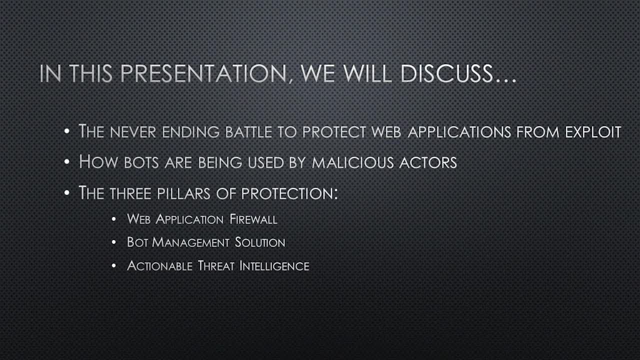 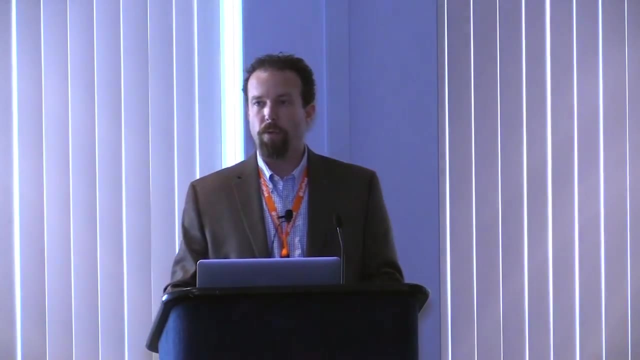 We'll also examine how bots are being used by malicious actors to up the game on their side. And then we'll go into the three pillars of protection: A web application, A web application firewall, A flexible bot management solution And then also actionable threat intelligence. 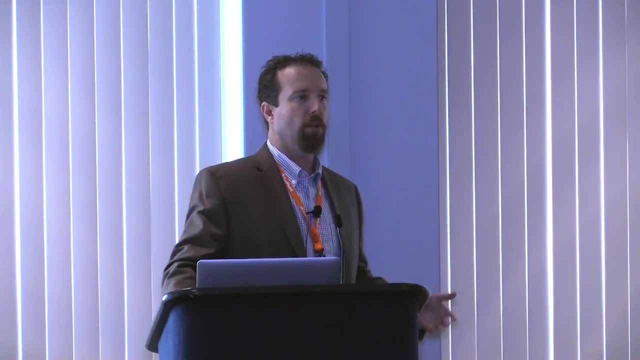 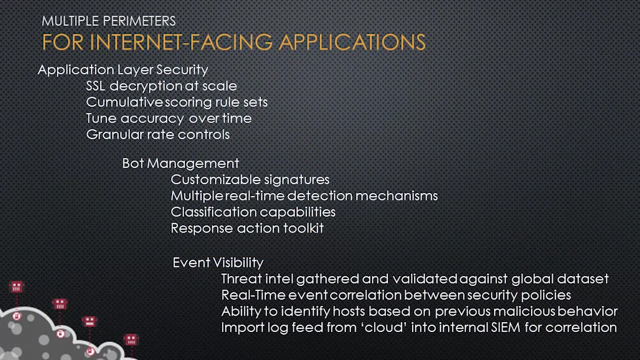 More specifically, when we look at securing our web applications, there are multiple perimeters that need different security tools. So, from an application layer security perspective, there are lots of things to take into account. So things like scalability. If you're in line, you need to be able to handle the SSL termination and decryption. 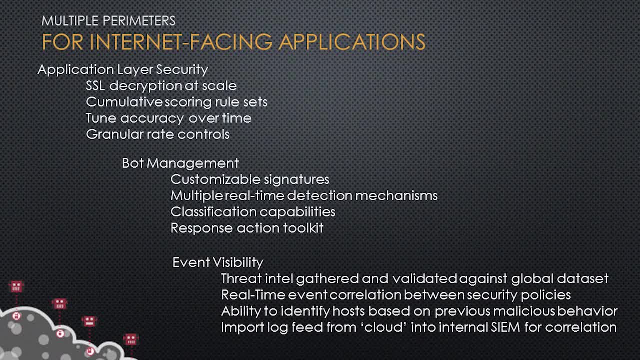 The cumulative rule scoring sets that give you an advantage over a flat, large rule set. Things like tunability- How can you maintain accuracy over time as threats evolve and so do your applications? Granular rate controls- These are things that are kind of a bonus from many people's perspective when you think of a web application firewall. 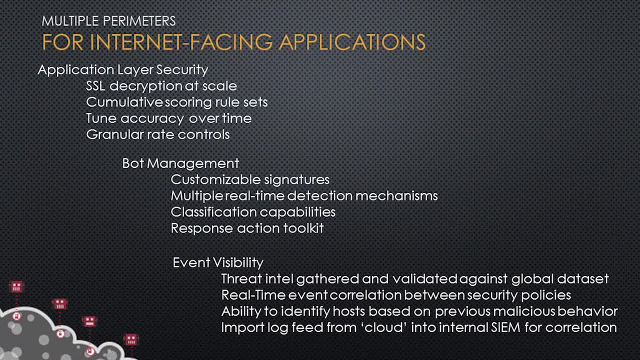 Having rate controls to also handle attacks against availability is a bonus. On the bot management side, Things like customizable signatures, The capability of defining your own signatures to incorporate in a rule set to protect desired bot traffic. Multiple real-time detection techniques, Catching the malicious, nefarious, more difficult to discover bots that are using up your web resources. 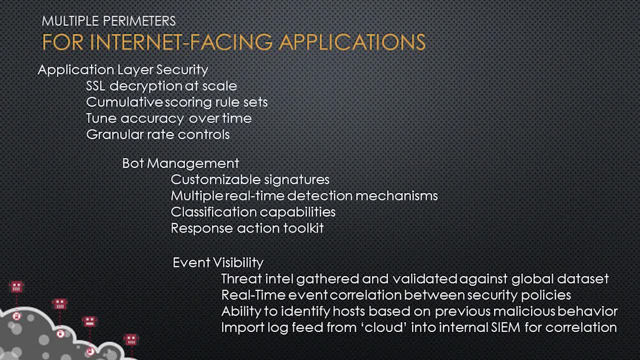 Classification capabilities so you can get a granular perspective on what your bot traffic is and then be able to apply different responses. So having a whole toolkit of responses To apply to those categories And, from an event visibility perspective, Having threat intel that's gathered and validated against a global rule set. 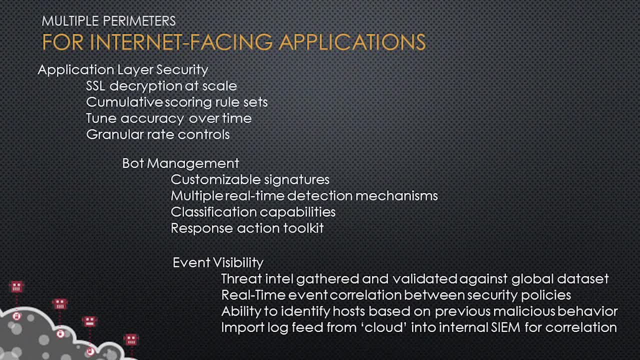 There's strong correlation there: Threat intelligence that is able to identify hosts based on previous malicious behavior And then give you the capability of taking action. The importability and applicability of that data needs to be both timely And flexible. So these are the three pillars that we will go through. 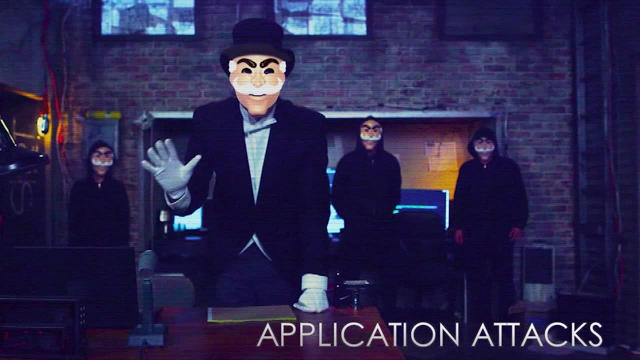 But first, as I said, let's take a look at the constant battle of protecting our web applications, And for this I have a few perspectives for you, Based on our global perspective. we gather a lot of data and we turn that data into consumable intelligence for our customers. 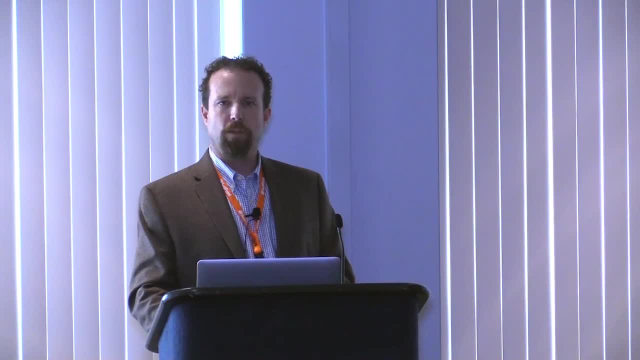 Monitoring for trends, looking at attack vectors, Looking for what's coming next Is part of the thing that we do, And we do that on a daily basis And provide that to our customers and to the general public. One thing we've seen consistently as far as web application attack vectors go: 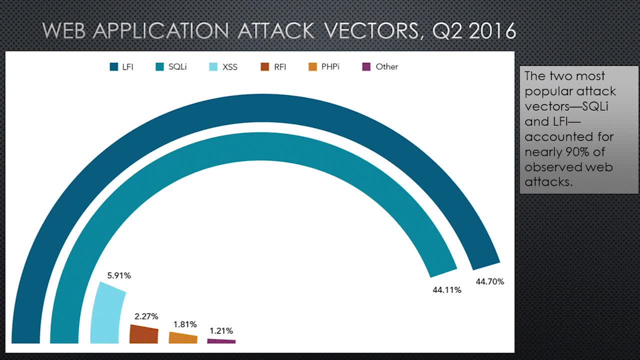 Local file inclusion and SQL injection are the top two attack vectors In Q2- in fact they were about 90%- are seen in about 90% of the web application attacks that we witnessed. Behind that we've got cross site scripting, remote file inclusion, PHP injection and a few other vectors. 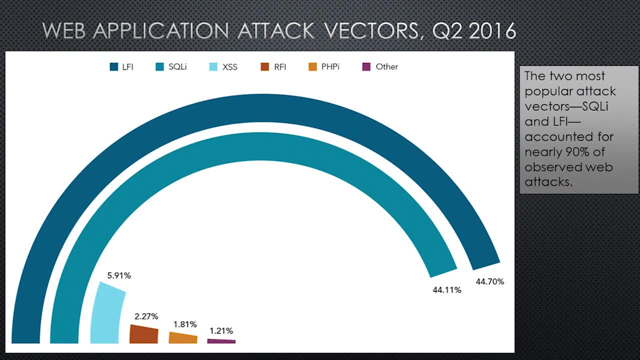 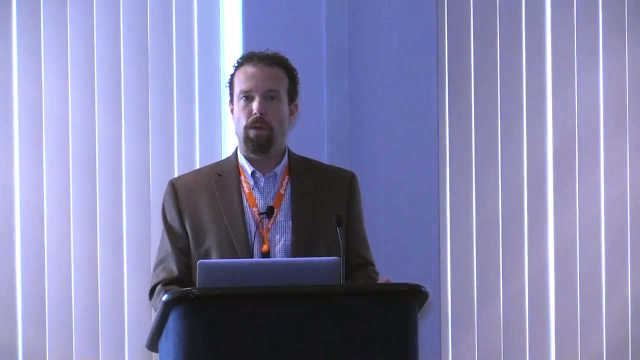 And they are just there. they're very well known. they're on the OWASP top 10.. They're there for a reason: because they work, And that's why we see so much use of these. For those not familiar with them, local file inclusion is an attack where the attacker is actually accessing resources that are already on the web server. 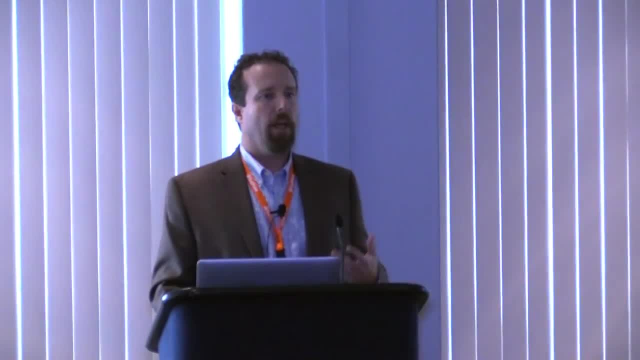 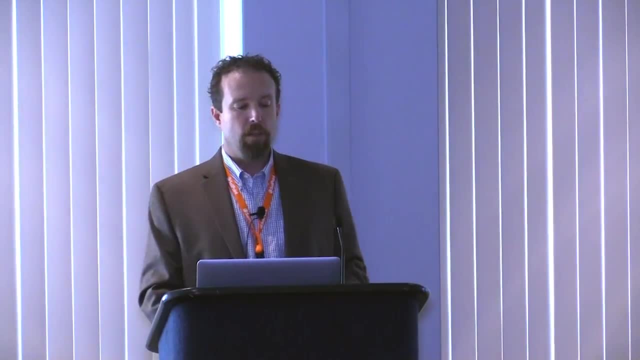 Through means that they should not be. So they're putting input in that's not being properly validated and therefore they have access to files and folders they should not. SQL injection is where your power is Passing SQL query parameters into an input field. They're not being properly sanitized and you're then able to exfiltrate data, execute administrative functions. 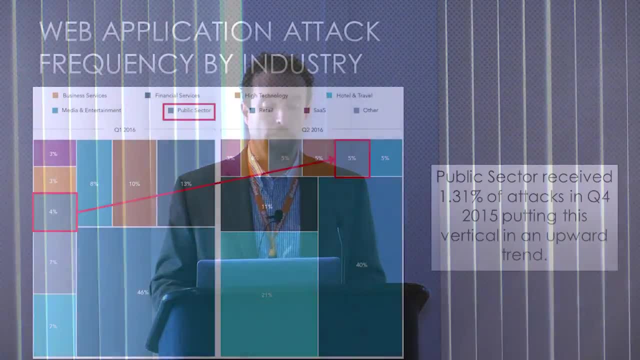 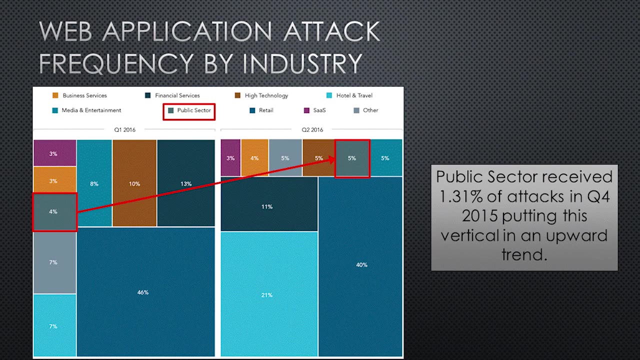 All things you don't want users, especially nefarious users, doing on your website. So who's getting attacked? We, like I said, track this data and analyze it from a lot of different angles. Obviously, there are some verticals that see a lot more attacks than, say, public sector. 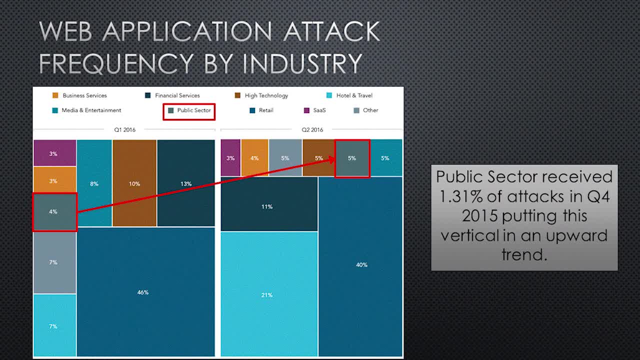 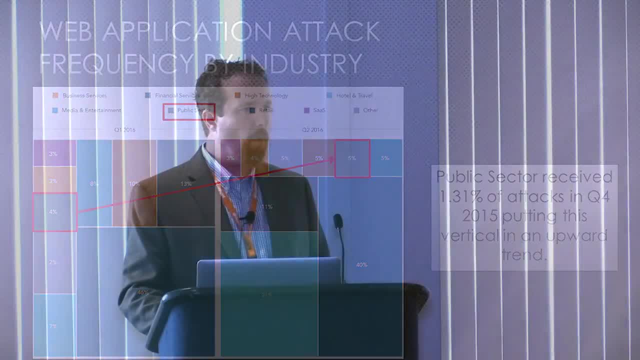 Retail financial services, hospitality, like hotel and travel- they see a lot of this But in fact when you look at public sector, last year Q4 we were at kind of a low of 1.31% of the attacks we witnessed were in PubSec. 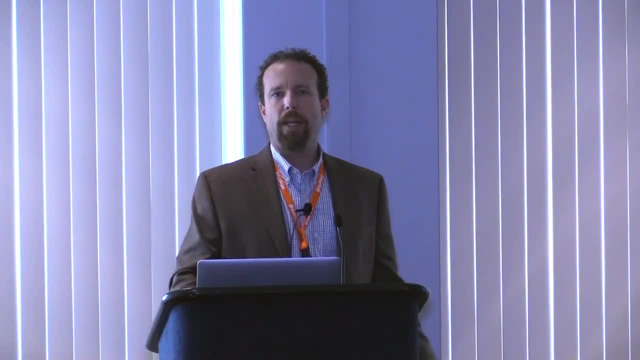 First quarter of this year that number went up to 4%. Then in Q2 it went up again to 5%. So it's definitely an upward trend now and when we look back a whole year to Q2 of 2015.. That number was at 9%. So 9% of all the web application attacks we saw a year ago were against public sector customers. That number went down to 7% in Q3 of last year and bottomed out at the end of 2015.. So a bit of a cyclical trend, like we see in a lot of things with security. 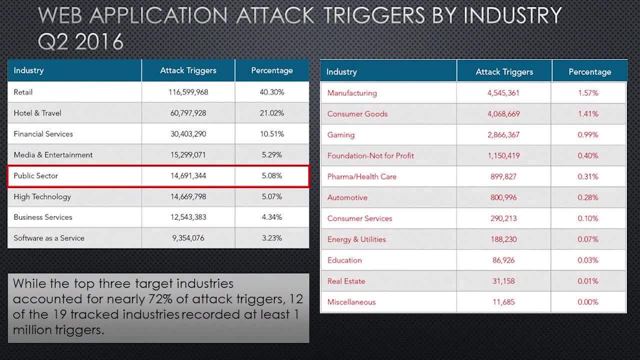 We don't just sanitize the data and present it as clean, neat, rounded numbers. We have all the specifics here and so when we talk about 5%, it's really 5.08%, That's nearly 15 million rule triggers we witnessed against public sector customers. 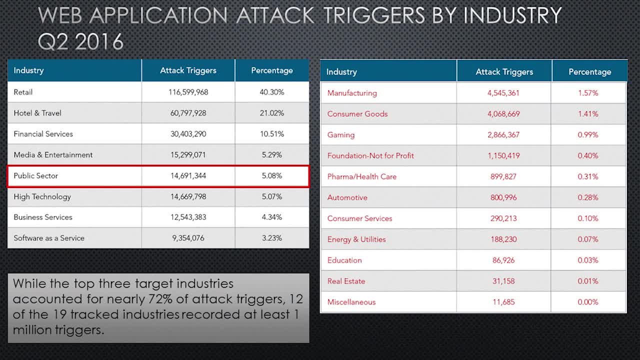 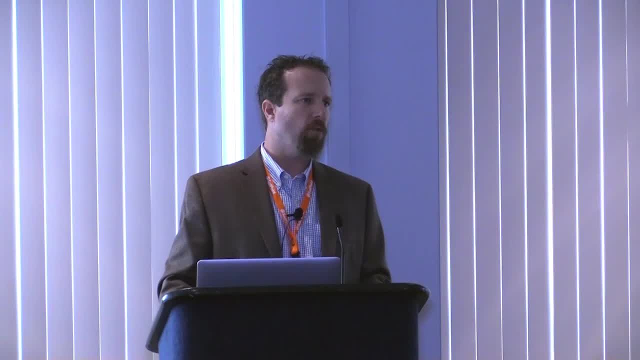 We also track the verticals that see even less, and that's important data as well, even though it's a smaller set, because many times we can capture and see future attack trends in these smaller data sets. So we manage all the data and we use that for our own intelligence. 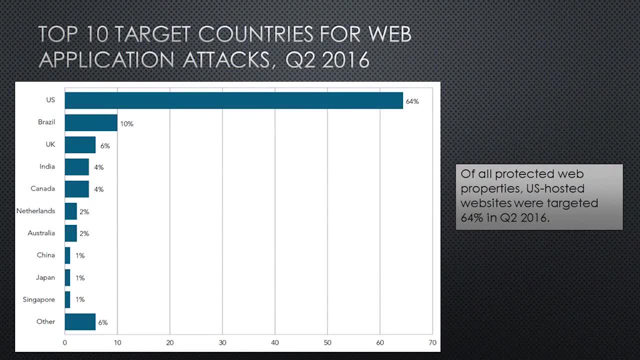 So who are the top targets? Who are the top targets from a nation perspective? It may be no surprise to most of us, but nearly two thirds of the attacks in Q2 were against US based targets. So that's where the resources are: A lot of companies, a lot of good information here, hosted within US soil. 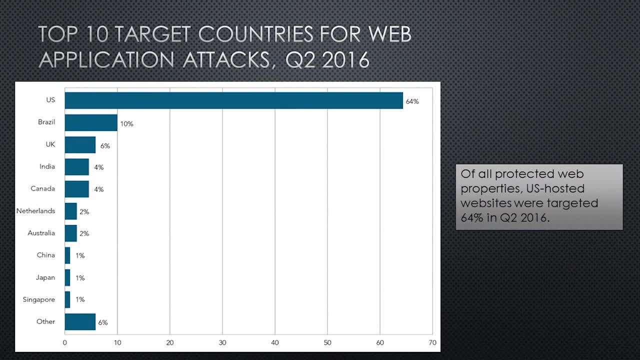 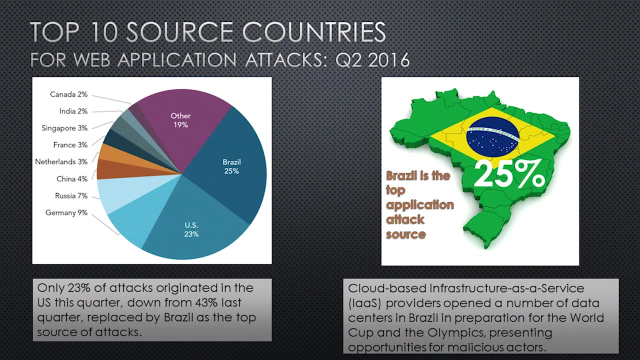 So we do see the largest chunk of those attacks, Brazil, interestingly though, with 10% of those application attacks in Q2.. That has been on the radar now for a few quarters And kind of going along with that, This is a new thing seeing a full 25% of the web application attacks coming out of Brazil. 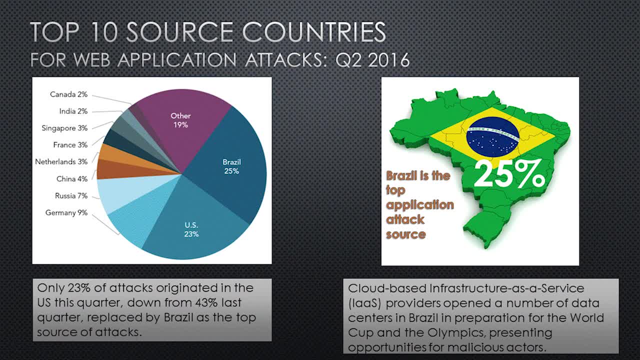 It's usually US and China kind of taking turns for top spot there, But Brazil kind of took over and started gaining more and more market share, if you will, of the source of application attacks a few quarters ago, Really due to some new infrastructure that came in there in support of World Cup, the upcoming Olympics. 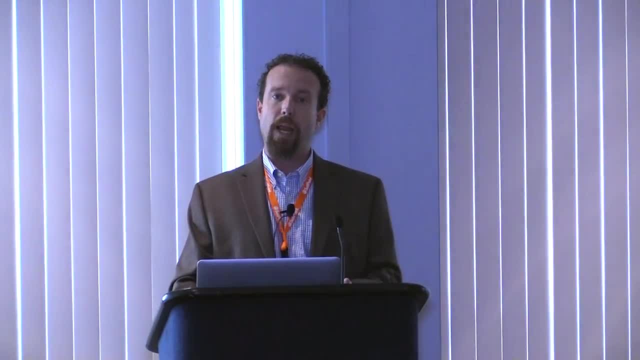 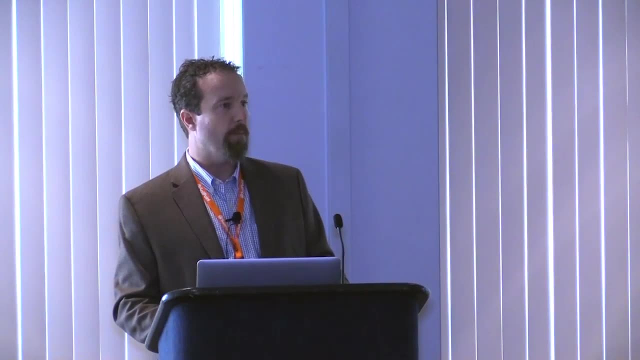 So these cloud infrastructure as a service provider started building out and there were then new opportunities for malicious actors to come in and exploit some of those resources They are attacking. obviously, with 10% of the attacks being directed at Brazil targets, They're attacking targets there, but they're also using that platform to attack targets globally and in the US. 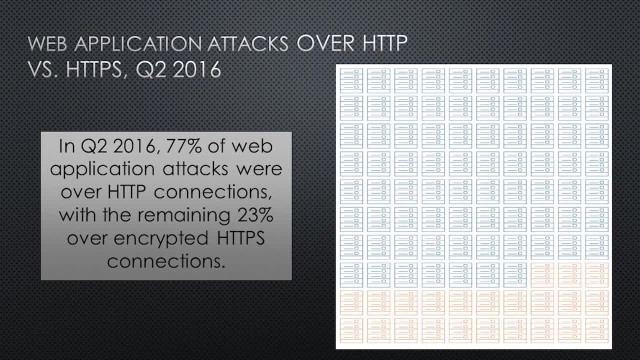 So over what medium HTTP HTTPS are they attacking? Well, about three fourths of the web application attacks we witnessed last quarter came over regular HTTP, Little under a quarter coming in on secure HTTP. I think it's important to remember when we look at this that HTTPS doesn't really protect the data in REST. 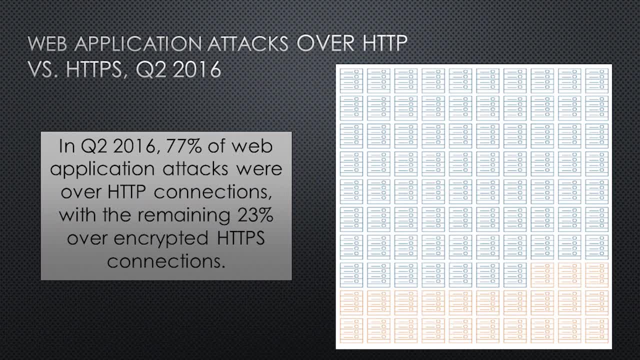 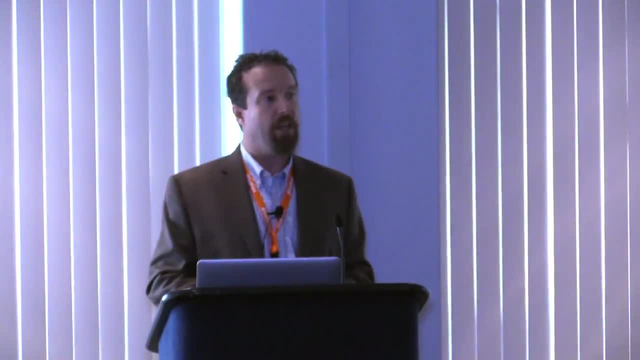 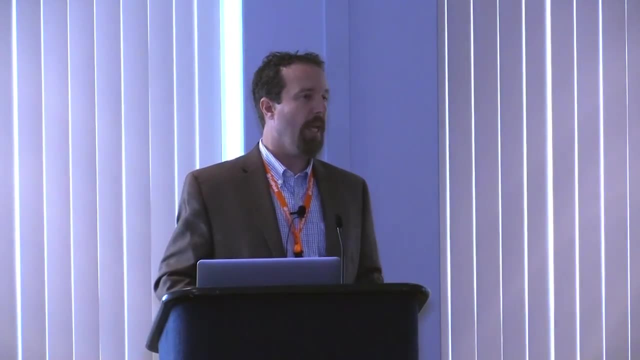 It's only protecting that data in motion, So that security is for your customers. It's up to us to secure that data once it's in our application, Once it's in our database, to secure that data at REST. So there's really no difference to the attacker if they can exploit a vulnerability in your application over. 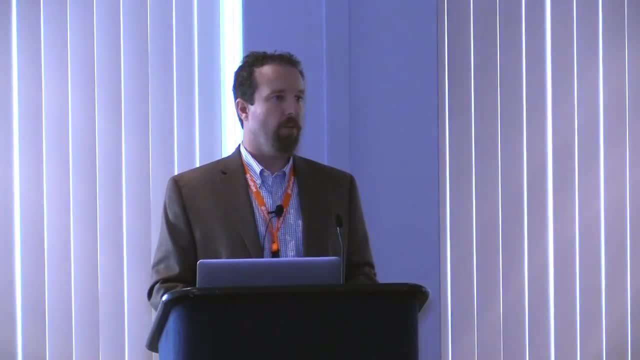 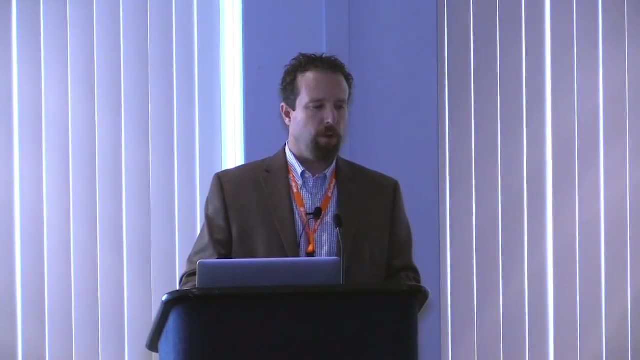 HTTP, they can still get the desired data even though they're not over an encrypted channel. Got an example here for you, with local file inclusion and SQL injection being the big heavy hitters as far as the attack vector breakdown goes. I thought it would be interesting to look at an oldie but goodie: remote file inclusion example. 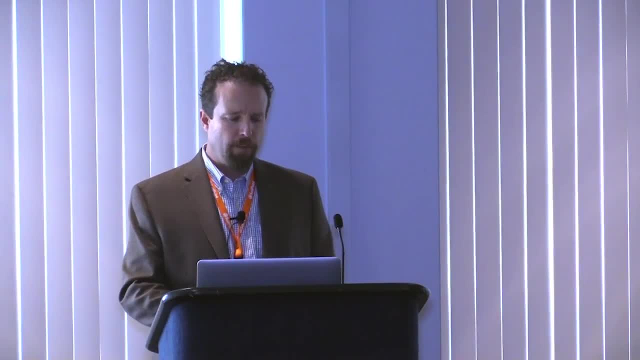 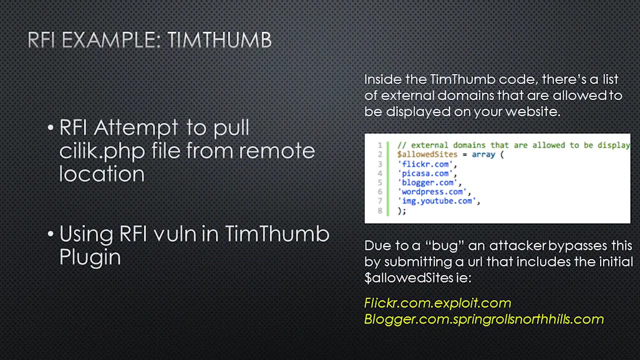 Remote file inclusion vulnerability is a type of vulnerability that allows an attacker to remotely access a file and bring it onto their targeted web application. OK, the vulnerability again occurs to non-validated user input. Tim Thumb is a great example of this, and it's actually a plug in that had RFI vulnerabilities as far back as 2011.. 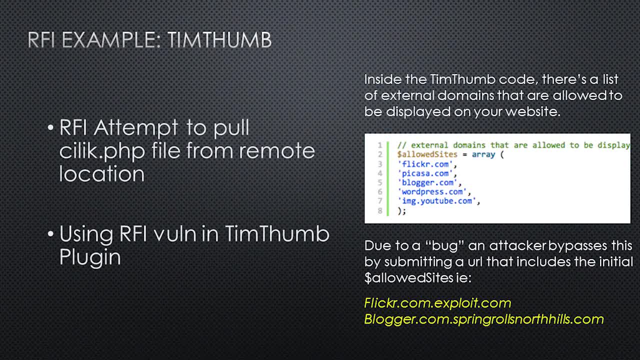 So that's why I said an oldie but goodie. This has been around five years, but we're still seeing it today. The Tim Thumb plug in allows users of a website to load an avatar on that site. So think of any web application where you have members, forums. 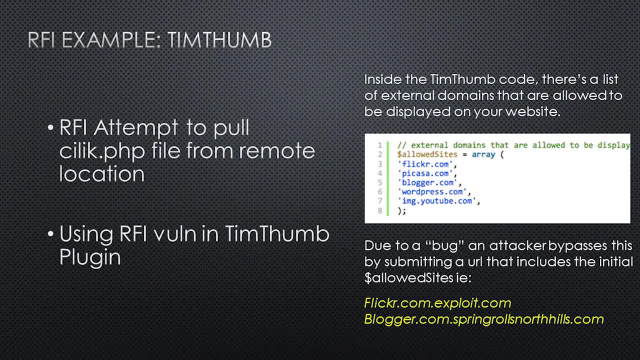 whatever type of thing. if you want to allow your users to customize their account and load an avatar, Tim Thumb facilitates that. What it does within the Tim Thumb code is an array, and you can see it on the right there where it lists out allowed sources of images from the web. 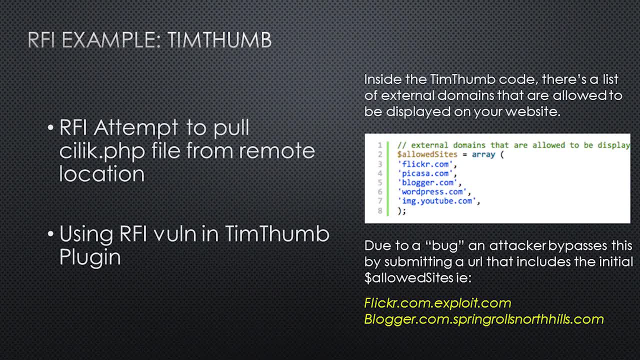 OK, that makes it easy, But due to a bug, unfortunately, the attacker only need reference one of those allowed domains in their URL input and then they can go to the domain of their choice. so they can then bring in files from other not allowed sources. 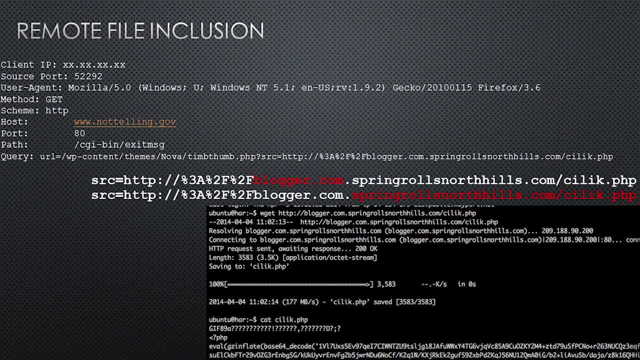 Those files, of course, aren't image files. They're going to be the malicious code that they want to upload on the web server. So we did see this. As I said, we still continue to see this vulnerability with Tim Thumb exploited. 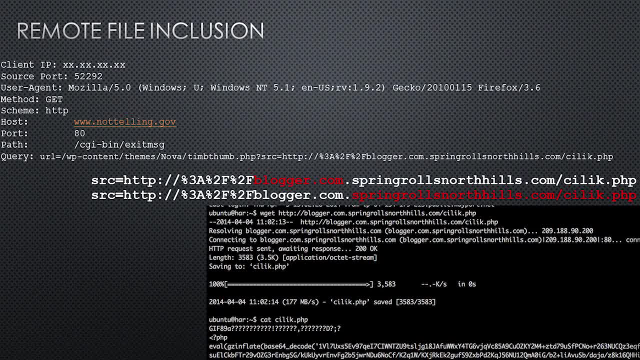 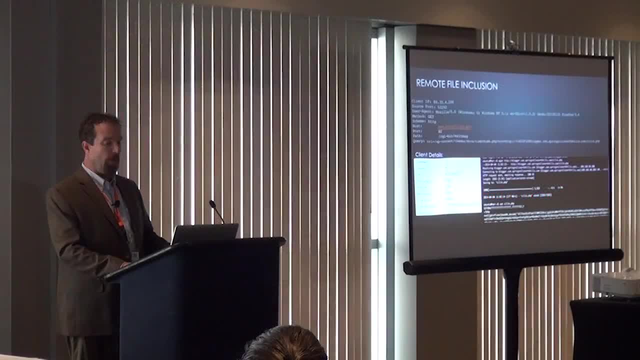 Recently we saw it with a government customer, And what happened was they used a version of WordPress that had Tim Thumb preloaded and it was a vulnerable version, and so it was attacked, And this particular attack that you can see a couple of screenshots. 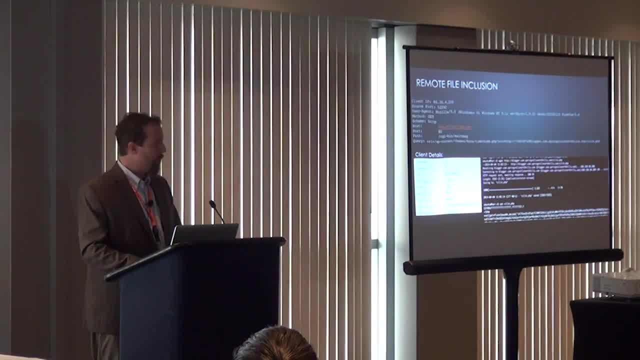 This one originated in Bucharest, And as you look at the query, I'll see if I can get my mouse over there. As you look at the query itself and go down this string, you'll see that they are referencing a website that they own. at the end down here. 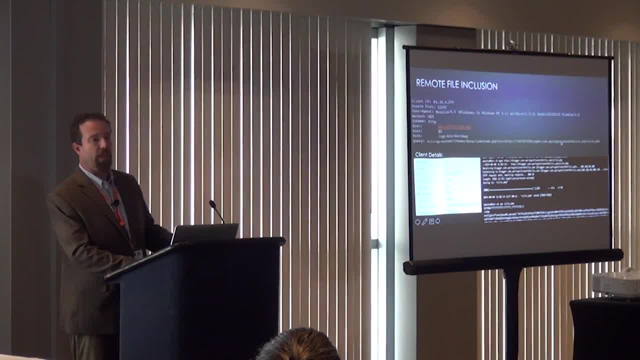 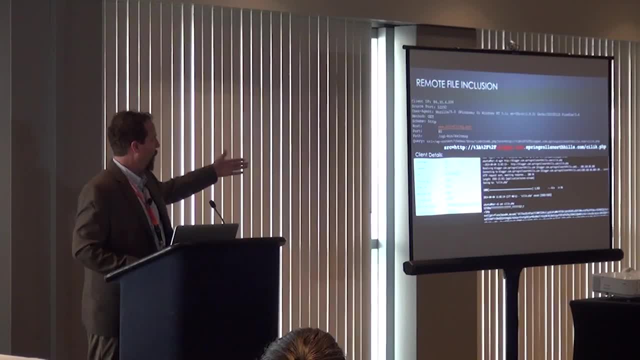 There we go, But within that, they are also referencing one of the allowed domains. OK, so when the Tim Thumb plug in focuses on this or looks at it, it's looking at bloggercom and it says, OK, this is an allowed source of image files. 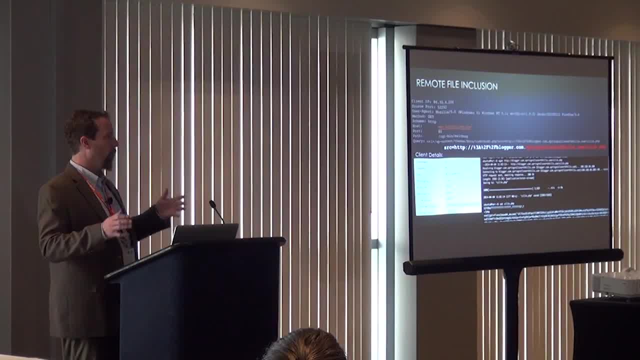 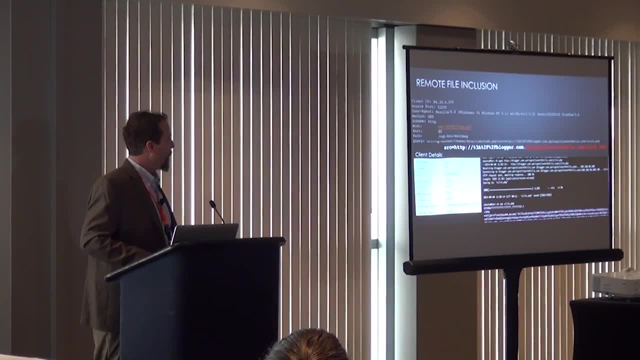 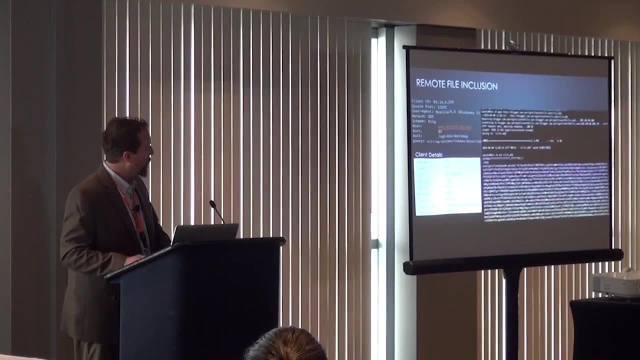 But what we want to focus on is the actual domain right before the final dot com. So bloggercomSpringRollsNorthHillscom is that URL. The path is SILICPHP, When we actually download and perform an analysis on this PHP file. 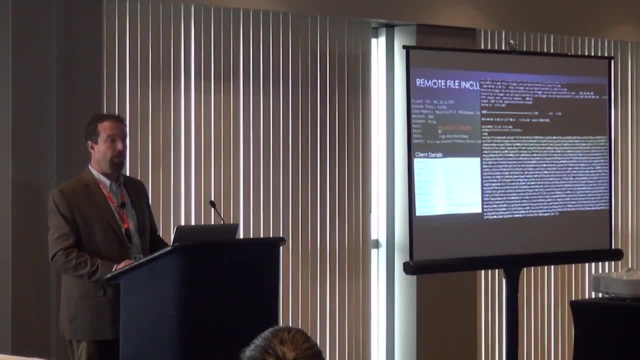 it actually has an image header built into it. If the administrator of the site has some content inspection on there for security and it's checking headers, it's going to say, OK, great, bloggercom image file. There's the header. Away we go. 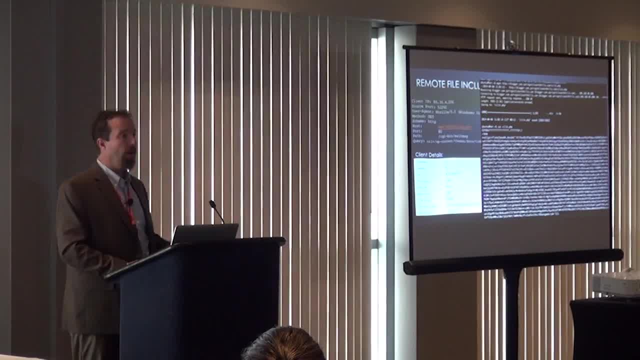 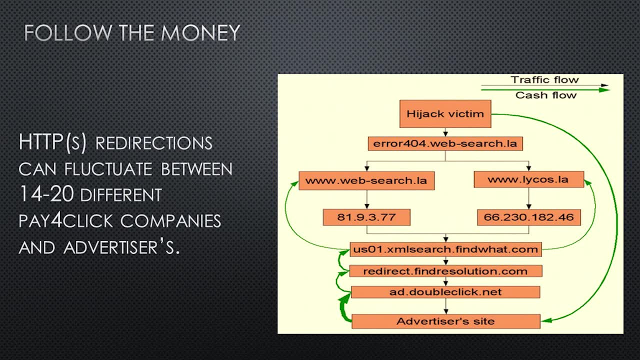 But in reality this is a base 64 encoded PHP file. that is definitely malicious. And what is it doing? It's executing a good old pay per click campaign. So once this file is uploaded on the target web server, Victim requests then are redirected. 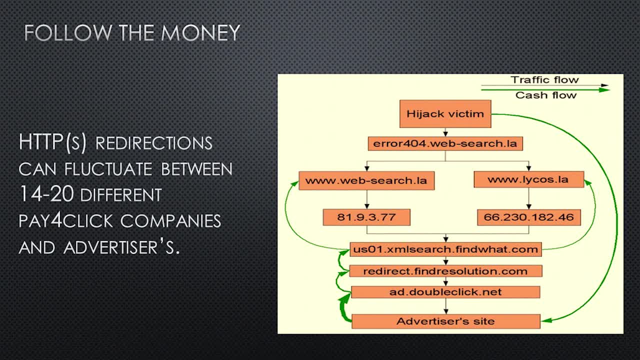 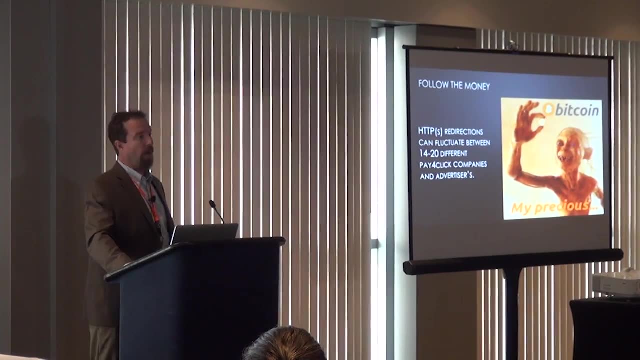 through a series, a multiple series in many cases. chain of pay per view ads, So the clicks are redirected. through this, The attacker gets the revenue very frequently. That revenue is going to be delivered to them with Bitcoin. Further obfuscating that attack trail. 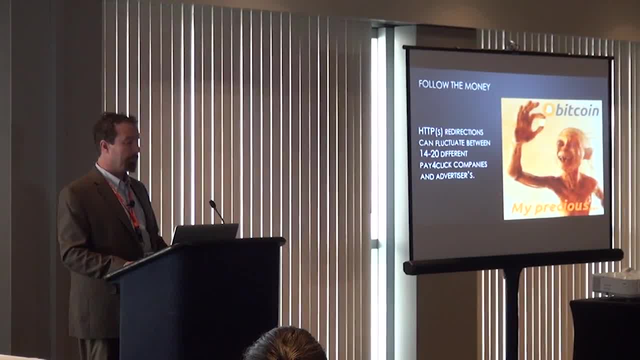 So they get the file on, they get the money. Nobody knows who they were. So just one example of how even all vulnerabilities are still exploitable. And so this is By having a solid web application firewall can help out with not only the old stuff. 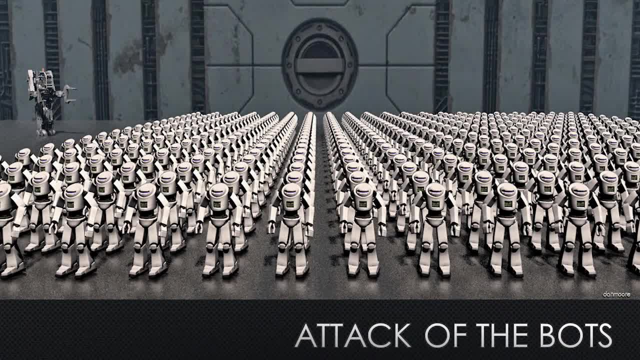 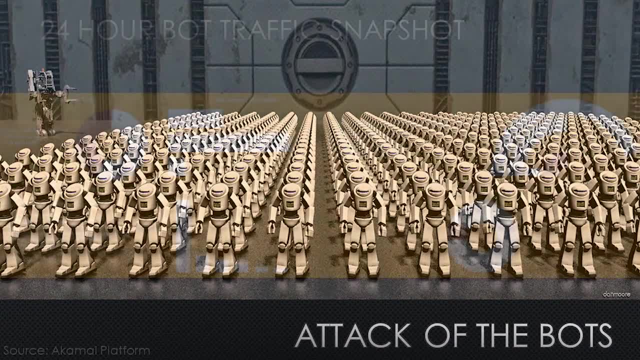 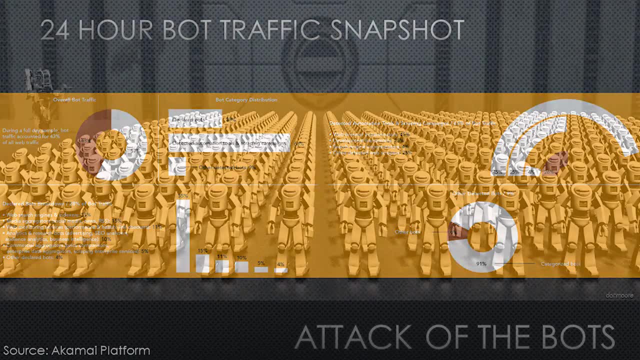 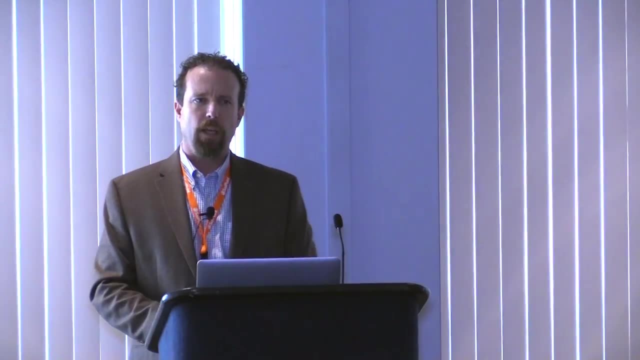 but then the new vulnerabilities coming down. Let's pivot, if you will, and talk about the attack of the bots. Actually, before we go forward, in case everybody's not familiar what we're talking about when we speak of bots With reference to the Internet and web applications, a bot is really anything. 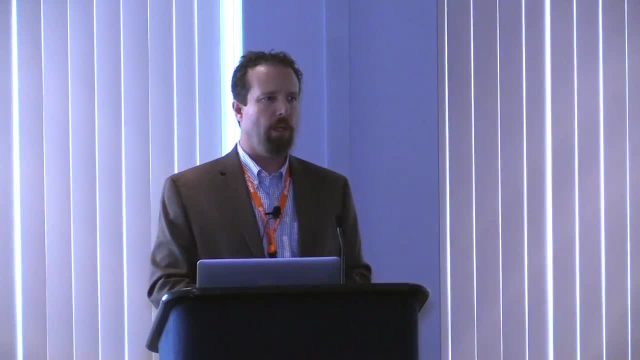 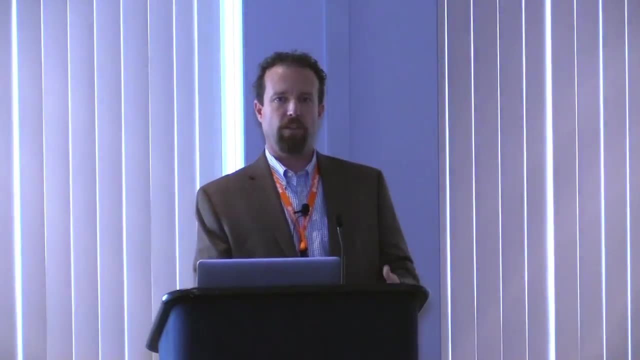 with your website. that's non-human. If it's a human, it's a human. If it's not a human, it's got to be a bot. So it's a software program and it can do good things. It can do things that you, as a site owner, want. 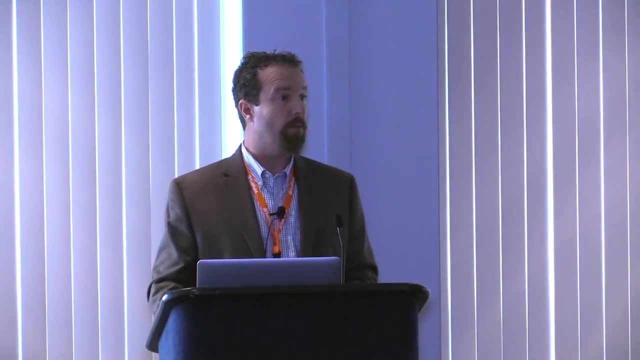 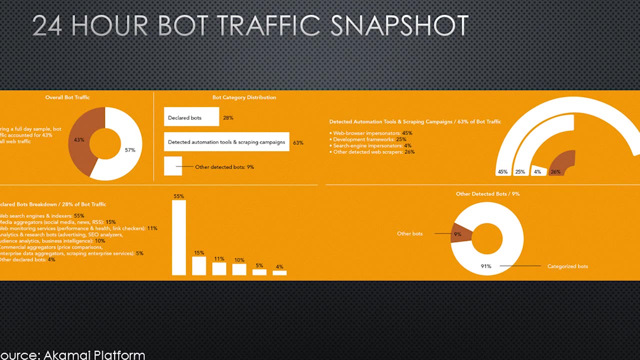 It can do things in the completely opposite end of that spectrum, Things you absolutely don't want. So to give you a perspective on how pervasive it is- and I know this is a small graphic, I couldn't figure out a way to make it bigger and still show- 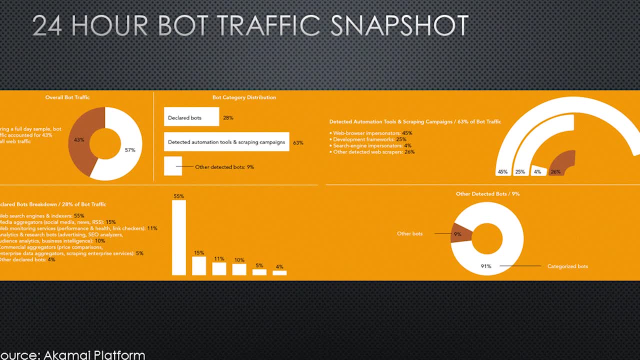 everything, but there will be a copy of this available for you. We did a 24 hour snapshot of all traffic on the Akamai platform and what we saw in that one day period were two trillion bot requests. They represented 43 percent of the traffic. 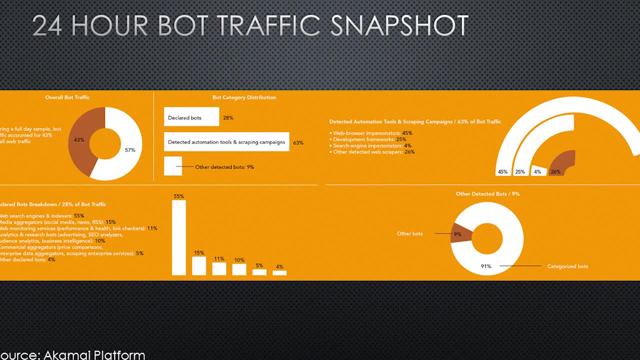 that day, And this is excluding bots that were executing overt malicious behavior, like executing denial of service attacks and actual web application attacks. OK, so excluding that, we've still got a large chunk of the traffic that's bot driven. Of that, 28 percent were declared bots. 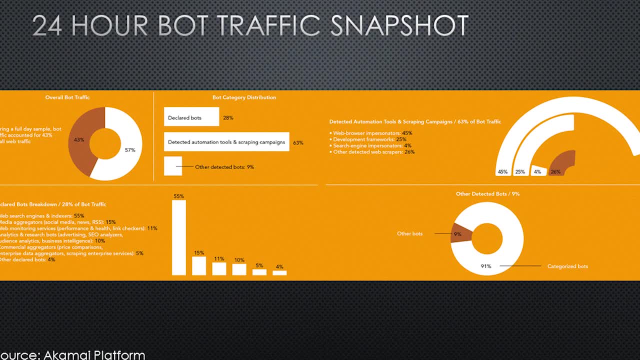 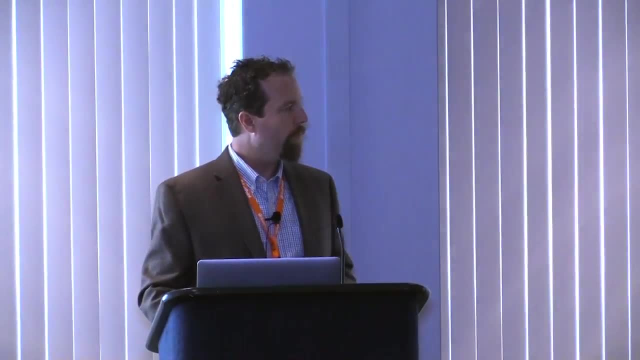 So declared bots are bots that are basically good bots. They're friendly, They identify themselves, You know their origin, you know their intent and they're stable bots And you can identify those with signatures. They do things like web search engine crawling, SEO bots. 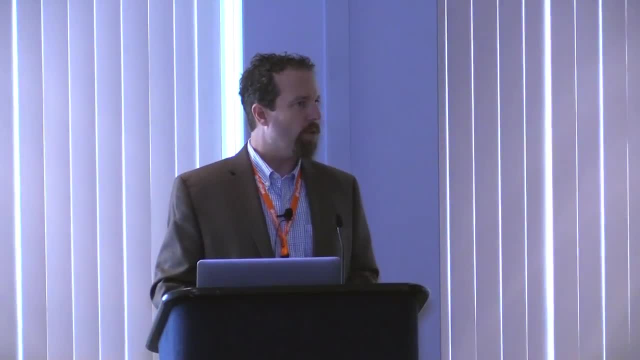 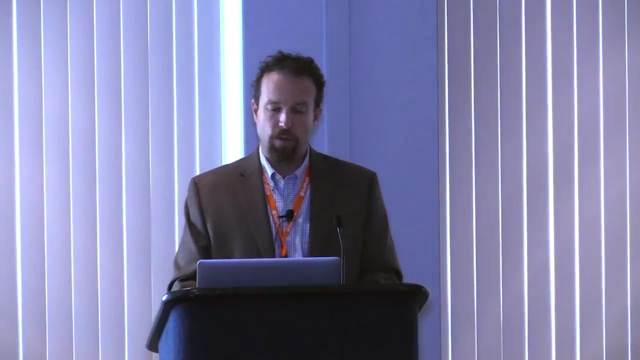 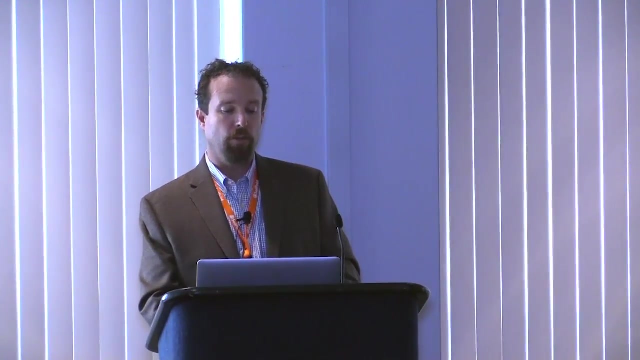 cataloging of data for data analytics- things we may desire. The next big chunk or the biggest chunk of data, however, were 63 percent of the bots, And these were actually detected- automation tools and scraping campaigns. So this category. compared to the previous 24 hour snapshot, we had done. 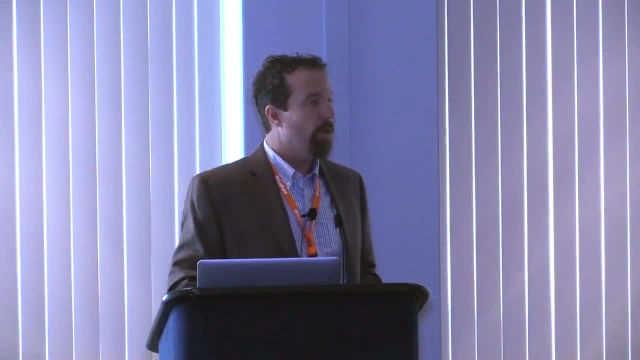 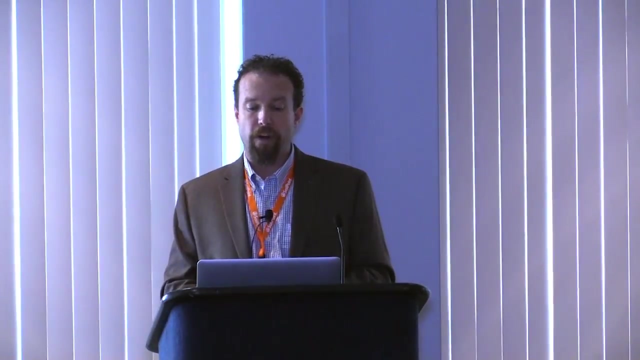 the previous quarter represented a tenfold increase. So these are the more malicious bots And what they were doing is more overt things like avoiding detection by impersonating real users, impersonating browsers, impersonating search engines, And they were engaged in more nefarious activity like aggressively scraping. 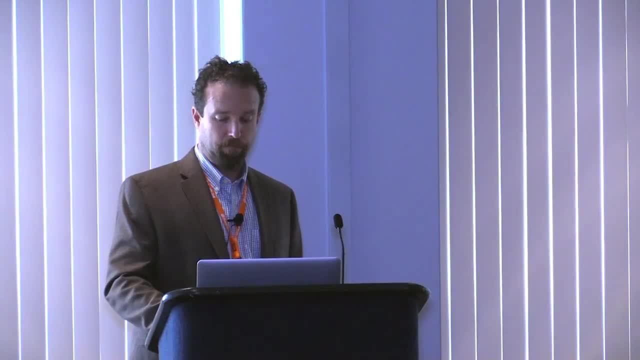 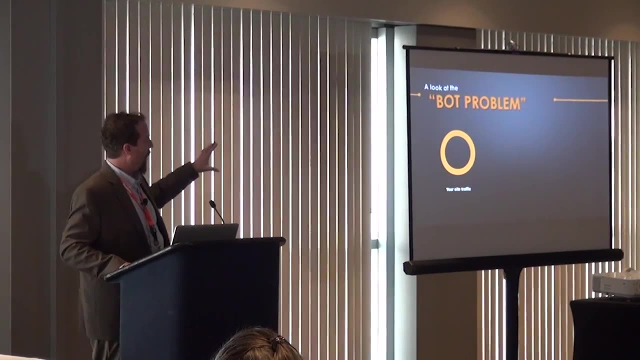 for fraudulent purposes. So, if you are the owner of a site or web application, this may be your view of the traffic, But when pushed, you may say, oh yes, well, the blue is our actual legitimate traffic. The red, however, that's our bot traffic, because everybody has bots right. 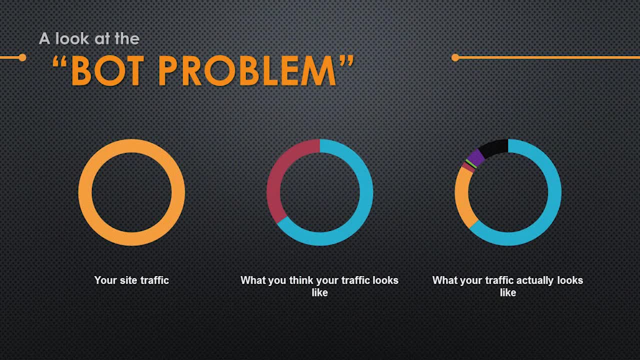 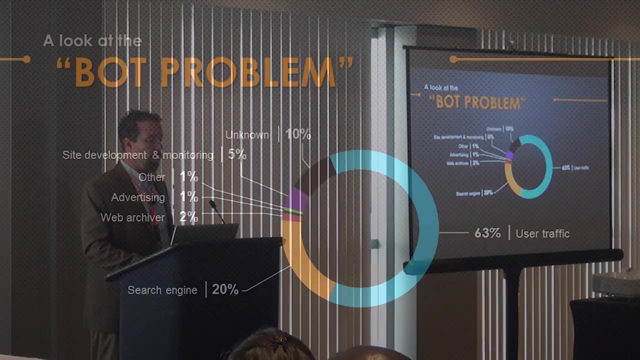 But that's still a big chunk of unknown stuff. Once you get visibility with a flexible bot management solution, you can start to understand what are these bots that are coming and making requests of my resources and what are their goals. OK, that visibility can then show you what portion of those of that bot traffic is. 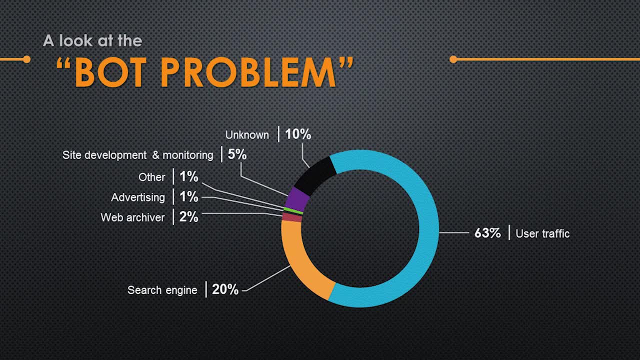 actually friendly bot traffic, things you may want and things you may definitely not want, Unknown bots that aren't detectable with signatures, And we rely on things like the behavior of their requests when correlated against legitimate user behavior, Anomalies- basically, transparent detection. 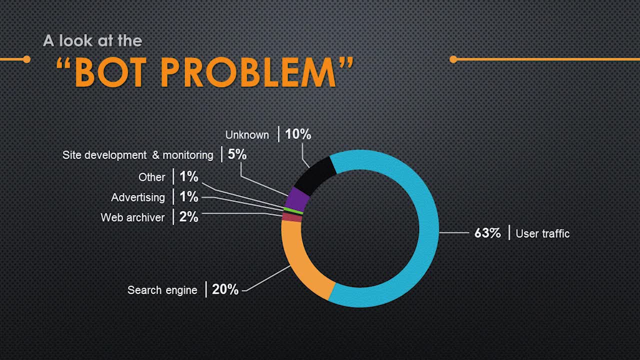 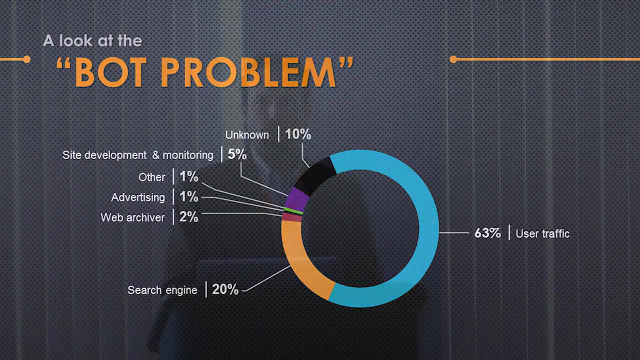 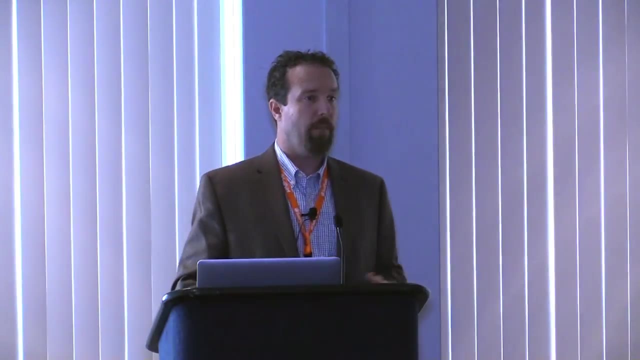 looking for various anomalies within those requests that indicate: this is part of an automated framework. this is part of, or originating from, a cloud platform- Things that real users coming to your site aren't going to be doing. I don't browse the Internet from a cloud VM, and I don't think many people do. 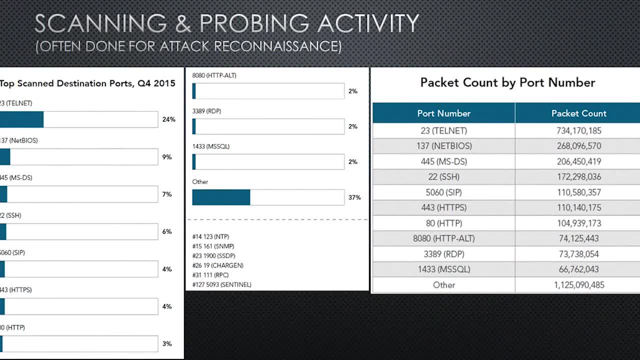 So what are the bots doing? beyond some of the good things that we think of with bots, They're doing some quite nefarious things, things that we can do as humans but bots can do more efficiently because they can work all day, all night. 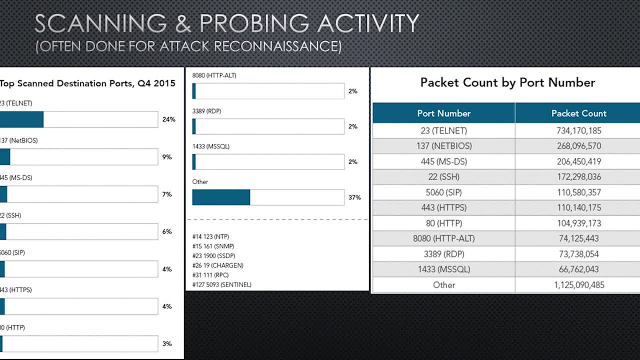 every day and execute scanning and probing type activities. You can scan larger chunks in a more distributed fashion by using a botnet than you can from single points, even going low and slow. So the data you see here is actually from Q4 of last year, where we gather a lot. 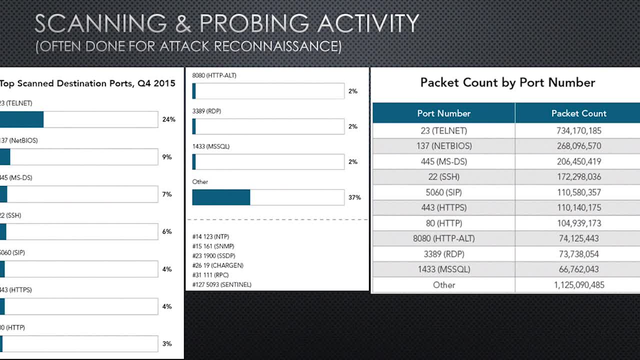 of this scanning and probing information and some of the top ports that were being probed, like Telnet, NetBios, MSDS. so Active Directory, Those are all good things to know if you're an attacker- And I see that you have an Active Directory port exposed on the public Internet- 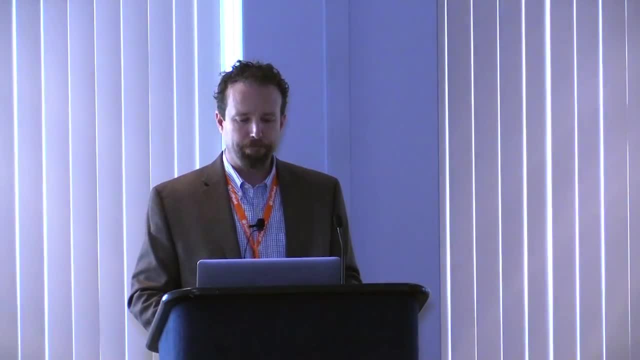 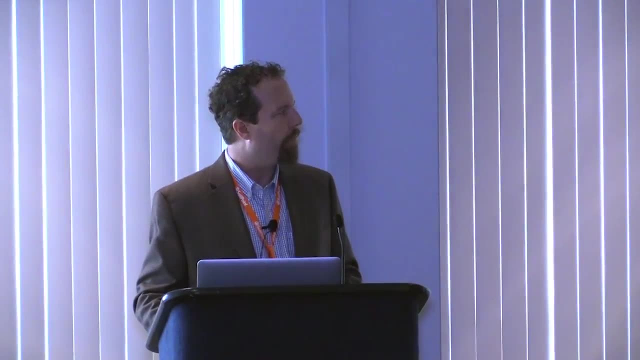 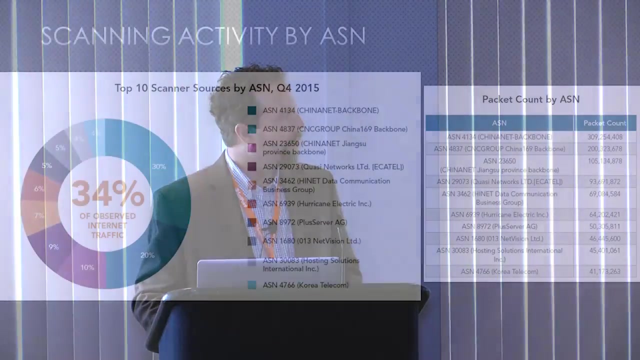 That information is handy and I'll be back tomorrow to check that out. Where was this attack traffic coming from? Because it truly is attack traffic. It's not executing malicious payloads but it's doing the reconnaissance. The largest three sources: 30%, 20%. 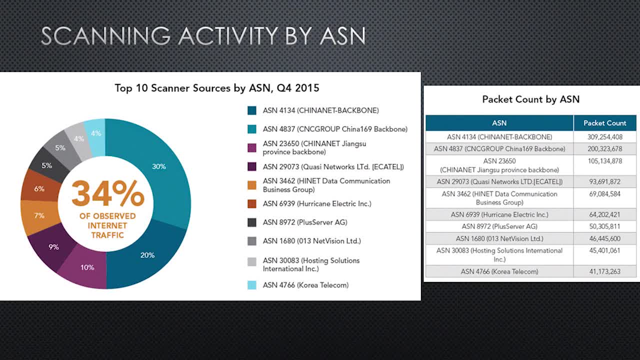 10% were all coming out of autonomous systems within China. So that's interesting intel for sure. We do see shifting patterns. as I said before, Historically we see a lot of the application attacks coming out of the US and China, but again we're seeing that shift now to other countries. 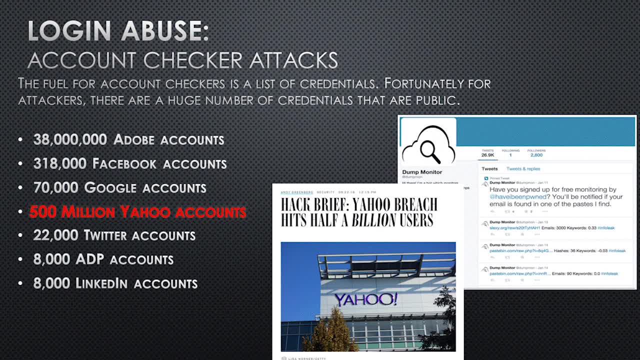 Another use of botnets, a malicious use, would be for login abuse, account checking. We're seeing more and more of this and again going back to the crux of the idea of why, to present these topics juxtaposed to you, Account checker attacks really rely on database dumps from big breaches. 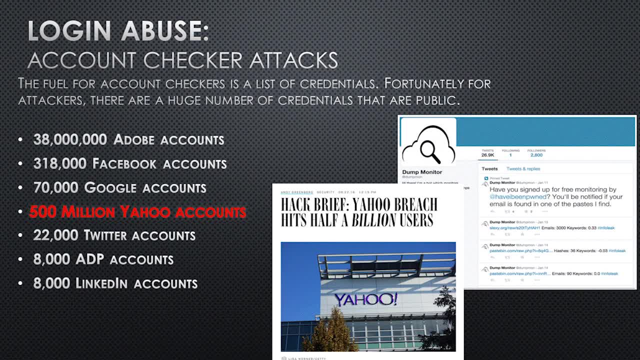 The breaches we hear about all the time. Breaches we hear about that kind of shock us 500 million Yahoo accounts being exposed. So I'm talking about username and password combinations. That's great data for that site, but they're probably going to rotate their passwords. 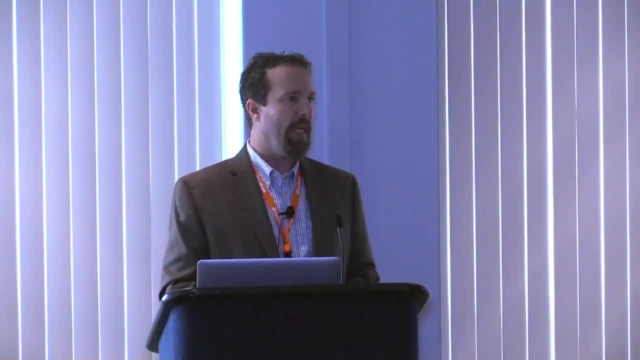 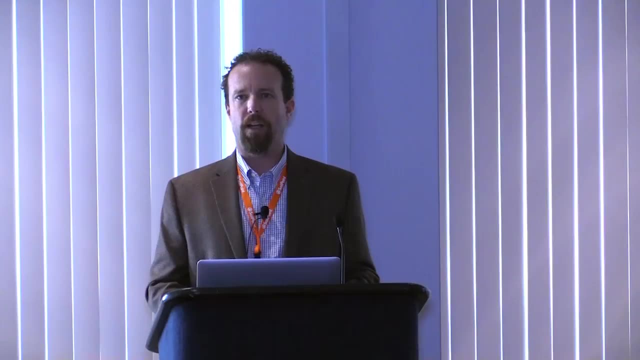 But how many people reuse passwords? Too many- And how many people's username is their personal email address? A lot. So account checkers take this data and they run it against other sites where they'd like to see if they have a valid account login credential set. 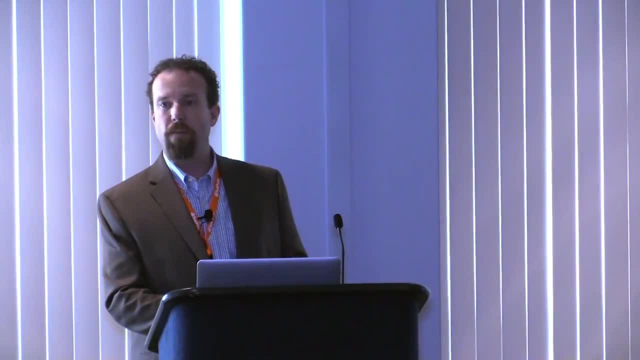 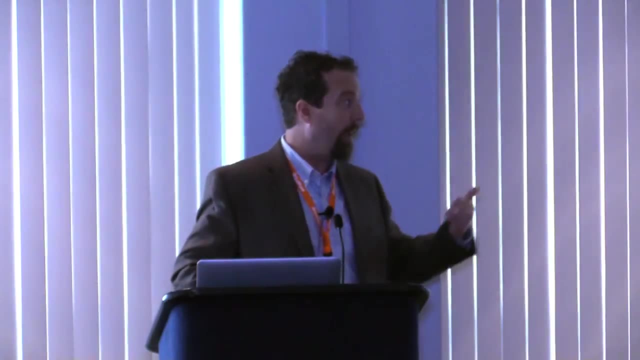 And so to do that, they use botnets, because they can do it in a distributed fashion. They can do it whenever they want, for as long as they want, rather than people behind keyboards trying to bang out 500 million account checks. So what are some of the techniques that are? 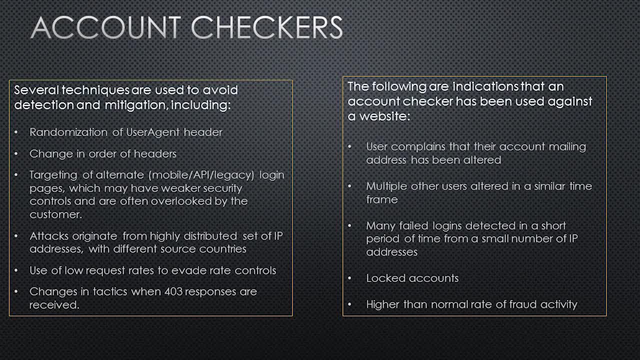 used by account checker attackers. Randomization of user agent headers and actually randomizing and changing up the order of the header fields in general. This helps avoid signature detection. Once you lock in they flip it around If I've got a thousand different user. 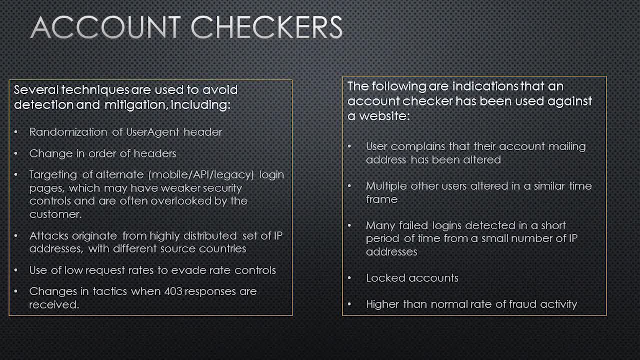 agent strings, it doesn't matter. even if they're all correct, You're not going to be able to lock in. if you're targeting the UA, They may target alternate login points, mobile legacy, API login or even the state ways. 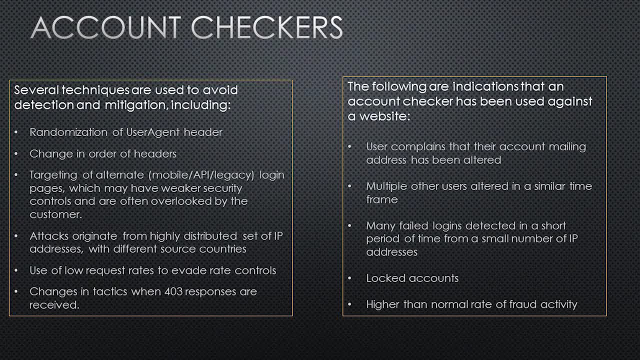 This was actually leveraged in an attack a little over a year ago. It was successful against a very large target, going after a QA login that did not have the security controls that the public login did. Account checkers are going to definitely use botnets and originate their source from a very widely distributed set of IPs. 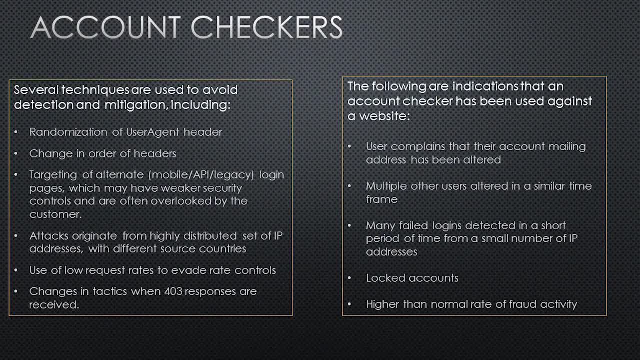 Global, if you will. You know, 10,000 IPs is a nice small data set, 10 million is more normal. OK, then they run these through proxies. VPNs come in low to low if they come in at 100 requests per second from a source that stands out. 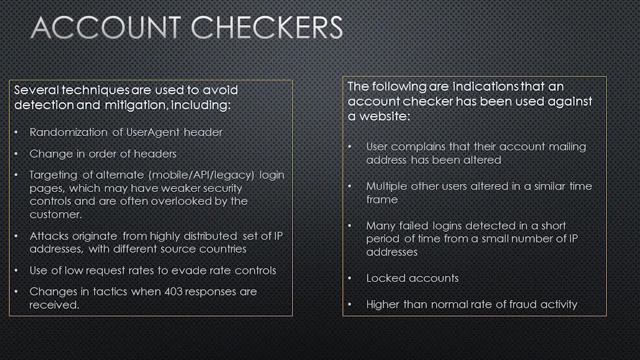 like a sore thumb. any of us can spot that in some log data. But if they're coming in at one request every 10 seconds, that's harder to pick up. But if you've got 10 million of them doing that, you're able to crunch through. 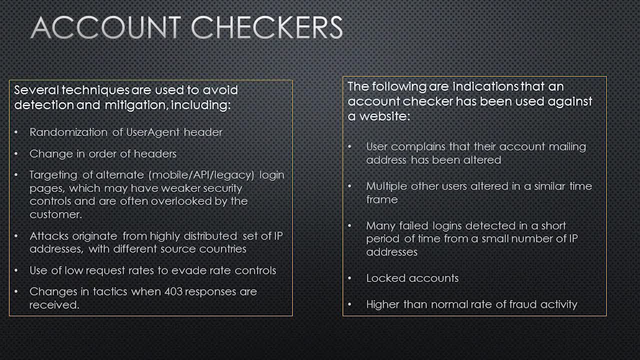 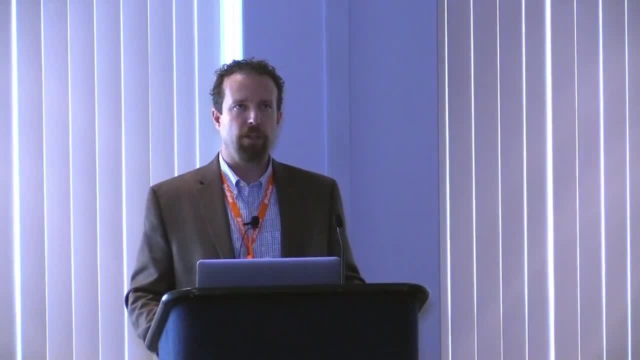 a lot of account checks in a very short period of time against dozens of different sites, then you have some more actionable data for sure. Another thing that they will do is there. you'll realize, in doing the tactical hand and combat against these botnet owners is that you are fighting against real people. 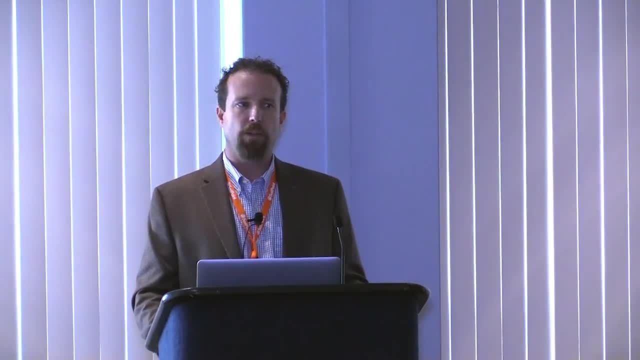 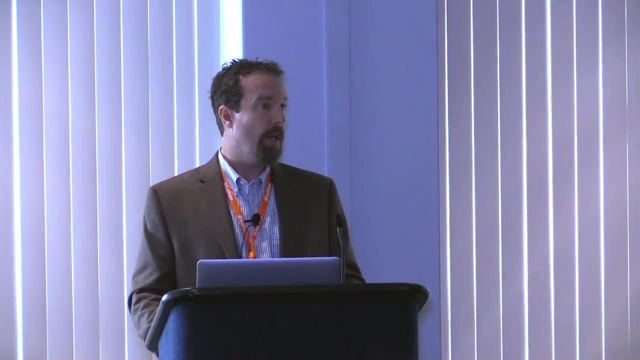 They've not done this, I didn't forget it. And when they detect that they've been discovered or you're locking on to them, serving them a 403 forbidden, they're going to change their tactics and they're going to come at you differently. I've seen individuals block based on source IP and it took less than an hour to jump to a completely different autonomous system from that botnet. So jumping to a different botnet, moving things around. Here are some indications that your application has been or is. 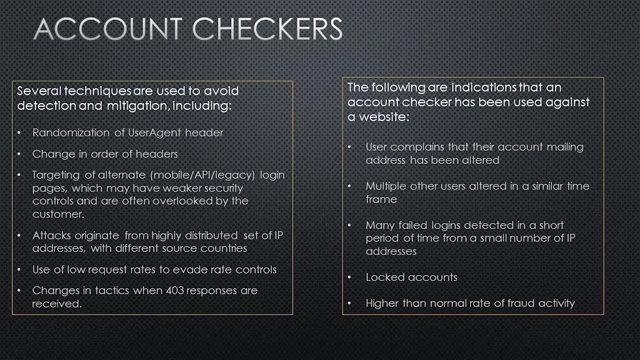 currently under attack from account checkers: Users complaining about changes in their account credentials. Example would be a mailing list. If they have any reason to have a mailing list on the site, suddenly that change. that might be an indicator. multiple other users. 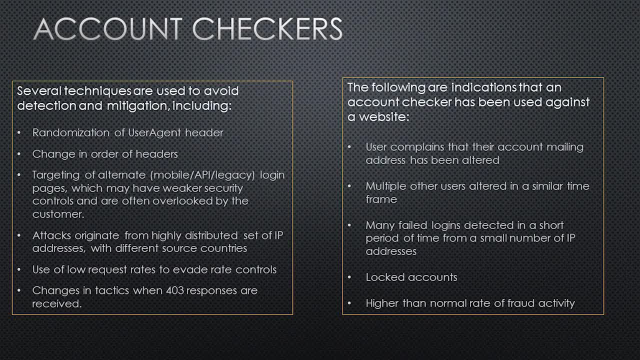 So you see a lot of users having alterations to their account in the same time frame. Similarly, you see a lot of failed logins in a short time period and locked accounts. If suddenly the phones are ringing because everybody's complaining about their accounts being locked out, that's a 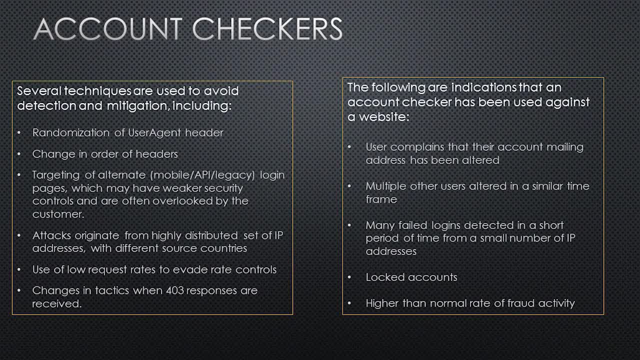 good indicator that your security mechanisms have kicked in and locked that account from too many failures. However, you're under attack And then higher than normal fraud rate. So if you're seeing actual fraud on a day to day basis, but there's an uptick, 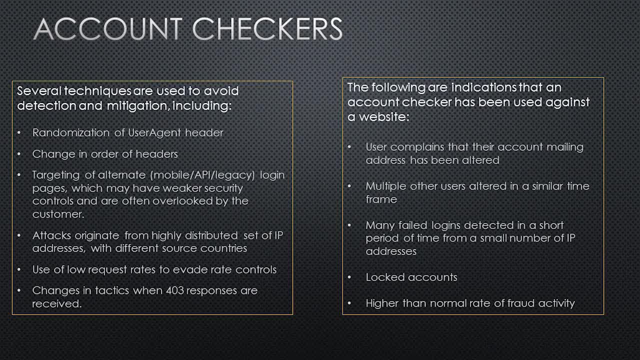 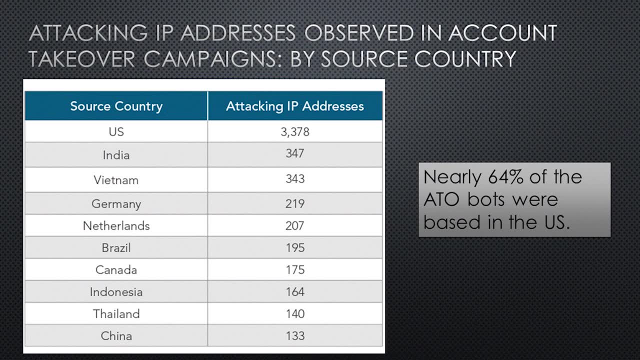 in that that account checking attack is well underway. We did document a case of account database theft against a customer last quarter and we took a small sub sample of those cases because it was again widely distributed And we analyzed a sample of 5300 IP addresses. 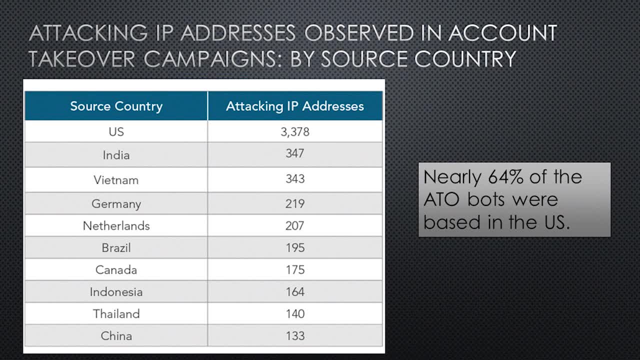 And what we saw were WAF triggers from the usual suspects that you would expect from an account database takeover attempt. SQL injection rules were firing as they attempted to dump on databases. Cross site scripting rules were firing as they were attempting to find footholds for phishing campaigns. 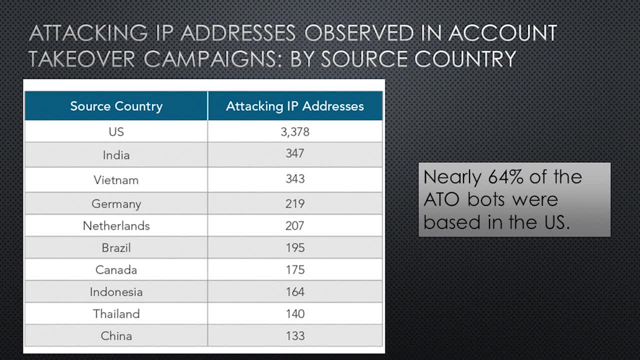 RFI rules would be firing in an attempt to potentially upload a web show. At the end of the day, we took this data, we had done the attack analysis for the customer, but we took it a step further and we said we now have intelligence about this attack. 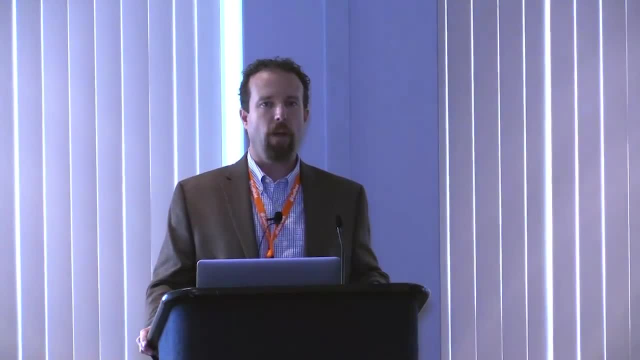 Let's see how far and wide it goes, And at the end of it we found that about 20,000 domains and subdomains had actually received malicious activity from this set of IP addresses in the last week. This affected the majority of the verticals that we do business with. 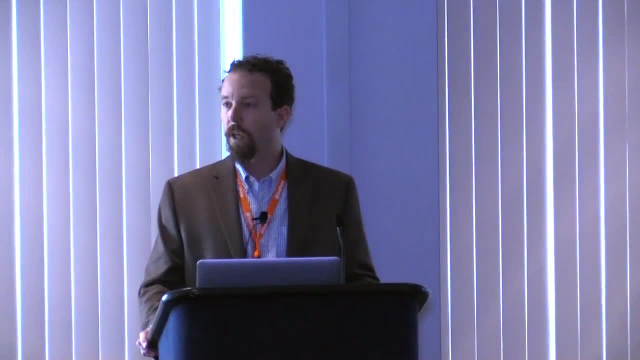 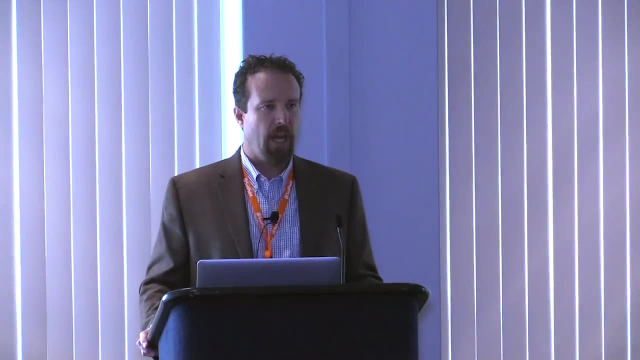 Especially focused in this case on financial services and retail organizations, But botnets are used for multiple purposes and they're not used once and thrown away. You'll see them in one attack, used over and over in other attacks, And that's where threat, intelligence and 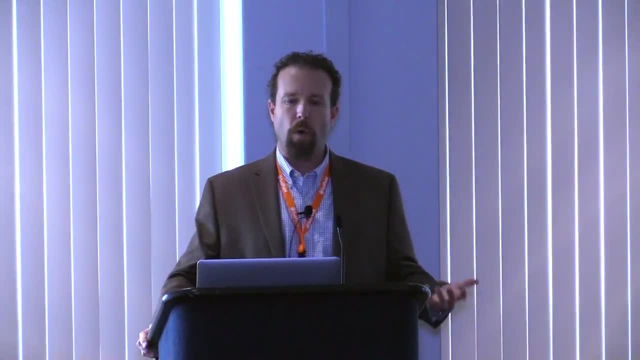 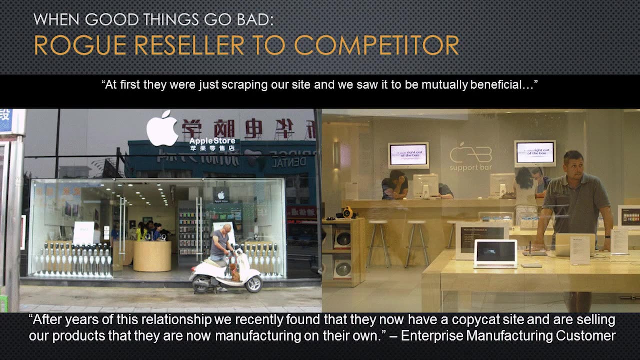 data about this activities come into play, knowing what's been going on in the recent past, And I included one more. I know this is public sector and this is a commerce slide, but you can't help but kind of chuckle to yourself. 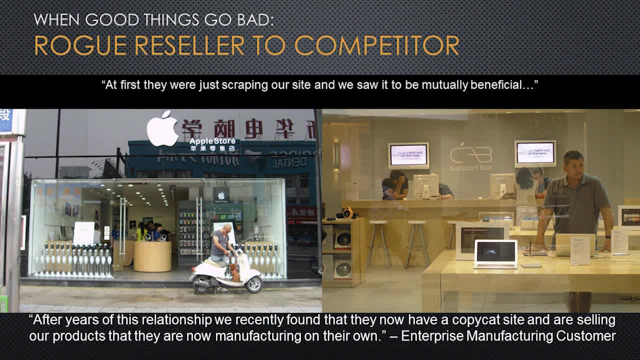 The sales teams might be OK with you know bots consuming your products. Sales are up, but you're losing customers And at the end of the day, good bots go bad when the bot operator actually opens up their own business and takes impersonation to a new level. 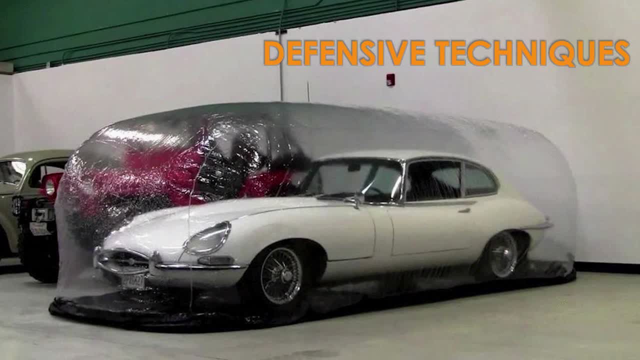 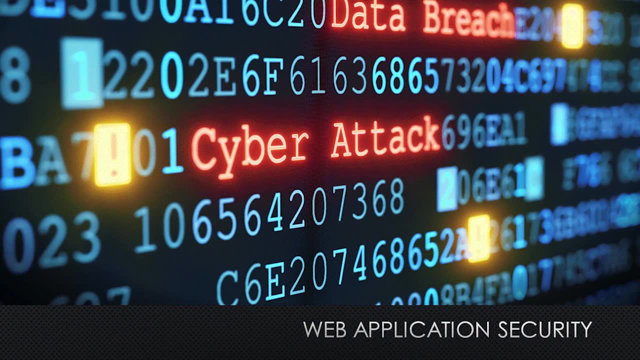 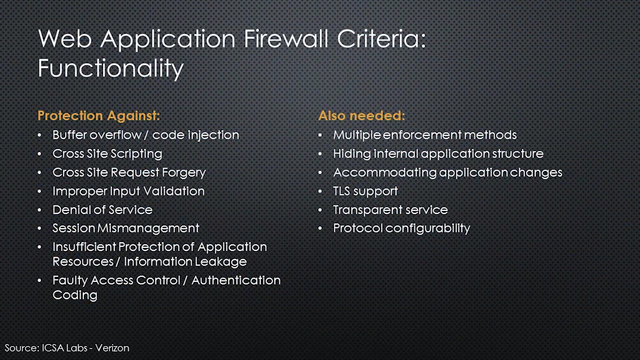 So what are some defensive techniques? So let's move now, if you will, into the three pillars and talk about web application security. We'll focus on first WAFs and some criteria. So when you start to evaluate your WAF or potentially implementing a WAF, 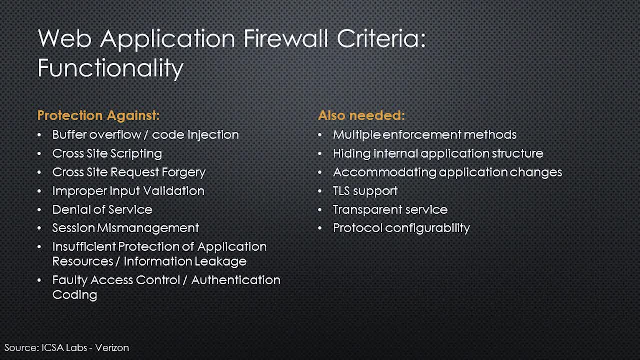 there's a lot of things to consider And first of all is: what is the functionality you're trying to achieve? And if you don't know what you're looking for, you won't know when you found it. I have here a list of some sample. 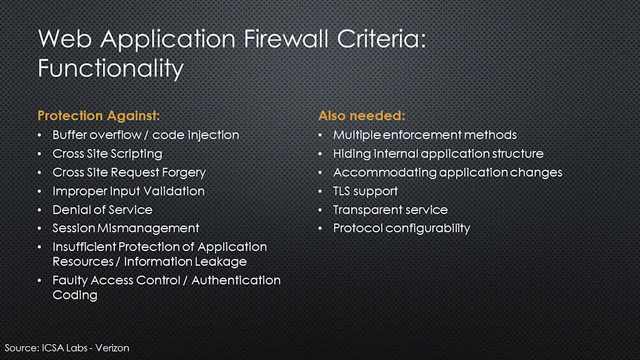 functionality protections that may be desired. This is from ICSA Labs out of Verizon, And they say you'll want your WAF to protect against things like buffer overflow and code injection, cross-site scripts protecting CSRF. so cross-site request forgery. 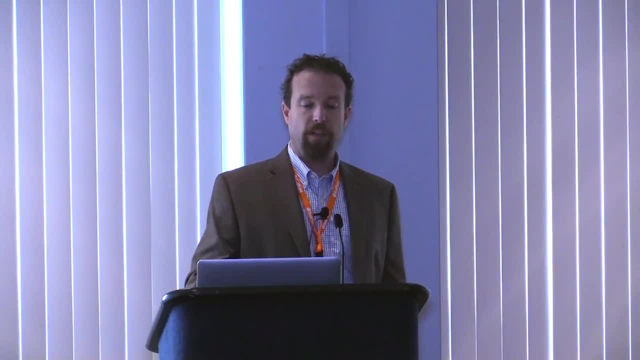 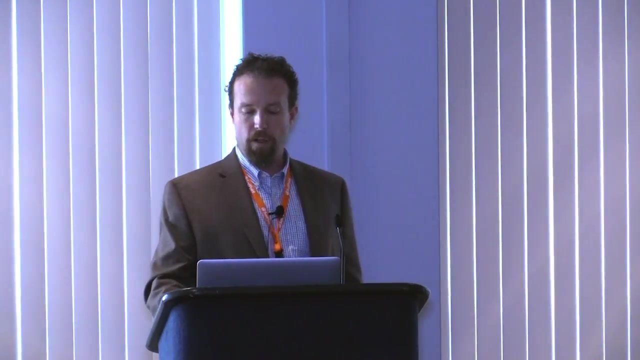 validation, input, DOS, things like that. A lot of that is OWASP top 10.. Good stuff right off the bat, But you can take it further with session mismanagement, insufficient protection against application resources and leakage, faulty access, control, authentication, coding. 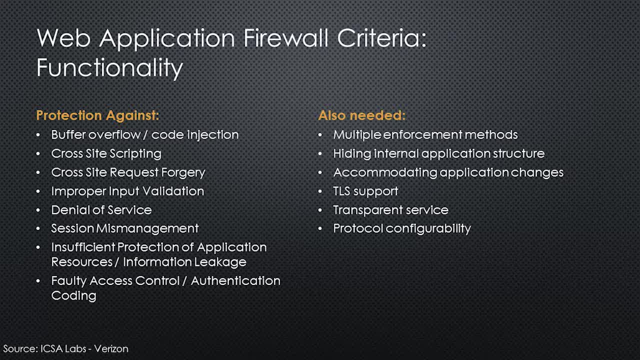 It depends on what your security requirements are for the WAF, but they need to be defined up front. You'll also need to consider other things like: what are the enforcement methods? negative security model, positive security model. Do you want the WAF to help obfuscate? 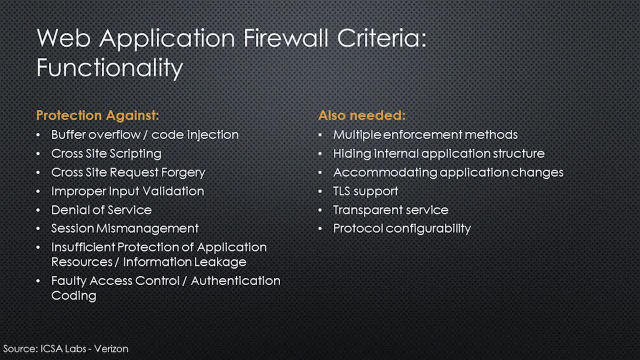 and hide the internal application structure? Probably yes. The WAF needs to be accommodating to change. It needs to be flexible and allow you to implement incremental updates to your security stance without having to increase your risk of exposure. So you need to be able to update it, test it and then push it into production. 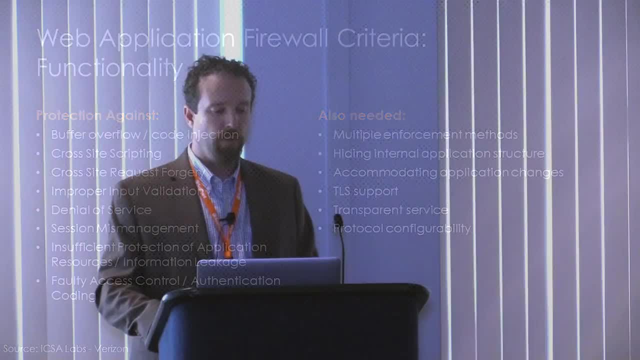 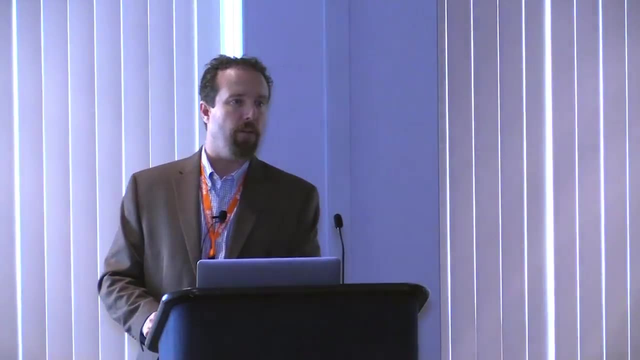 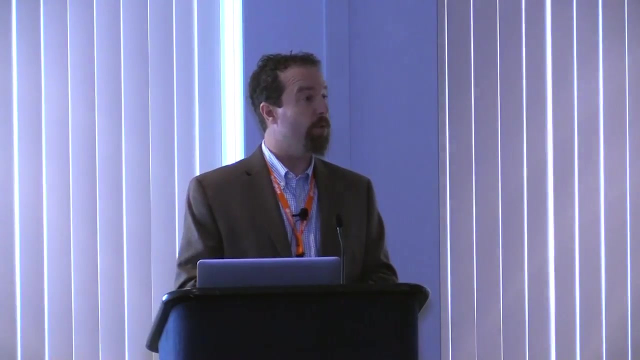 all the while maintaining the current posture you have. TLS support is included here, because if it does not have TLS support, it's going to have to be offline, out of the path of that secure communication, And when you're out of line you're just merely an observer. 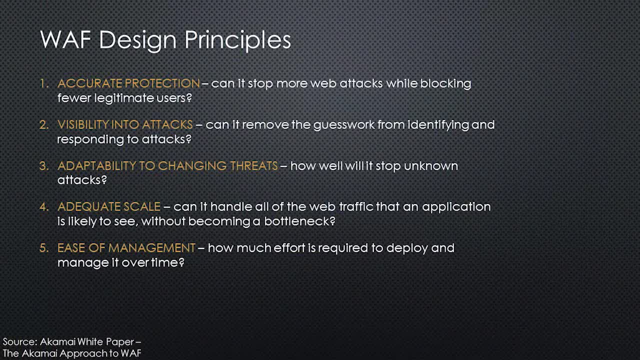 Okay, let's move it up a layer and look at it from a design principle perspective. I think these are five solid design principles for a web application firewall. So accuracy, accurate protection. Can you stop more web attacks while not blocking legitimate users? 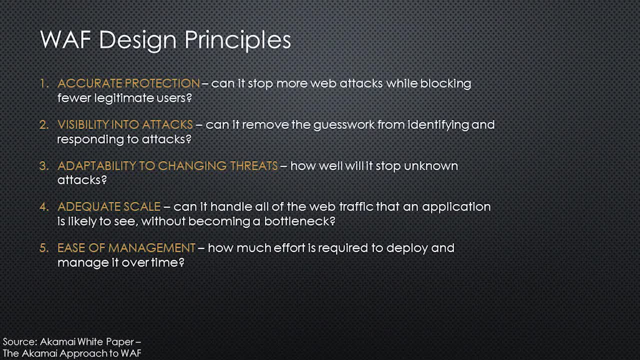 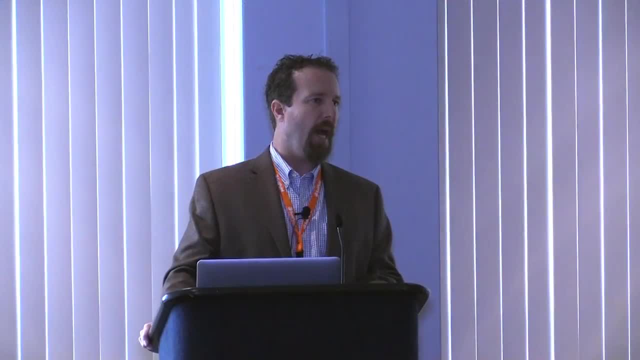 Okay, very important. So it's number one. What is the visibility that the tool affords you? Can you, using the tool, determine what were the triggers in deny actions? You need to have that perspective to understand again how well your security. 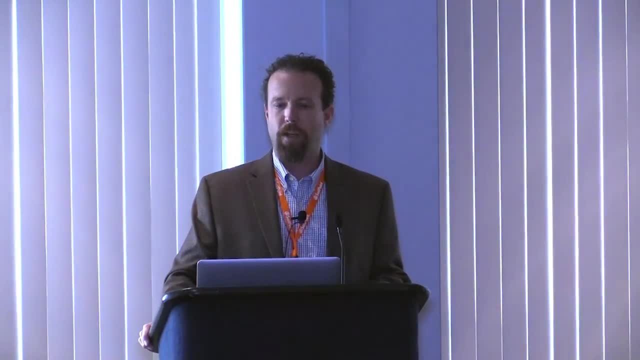 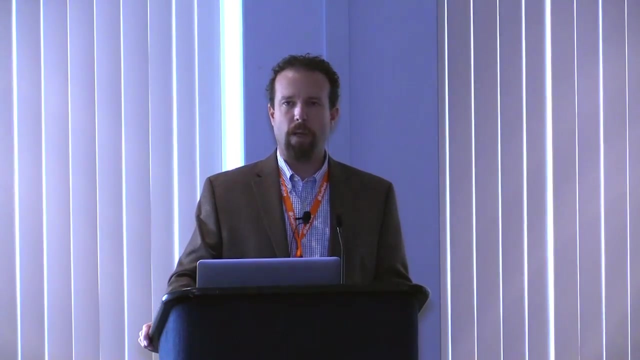 configuration is performing and are you contributing to false positives and blocking legitimate users? Adaptability to changing threats. How will it stop the unknown attacks? This is important because you can't be chasing CVEs. That is not a way to go. Definitely, there are some that you have to make something customized for. 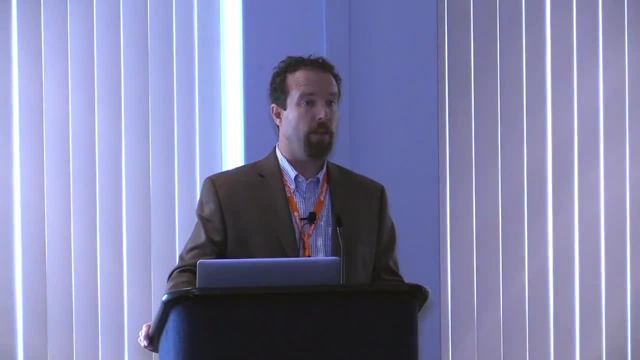 But at the end of the day, if you're chasing CVEs and trying to stay in front of it with that type of a security model, you're going to need another full time employee or two or three on that staff Number four- adequate scale. Kind of basic here, but can it handle the load that you're going to put on it? Can it handle more than that, Because it's probably going to see more than that? Can it still perform under attack? And finally, ease of management. 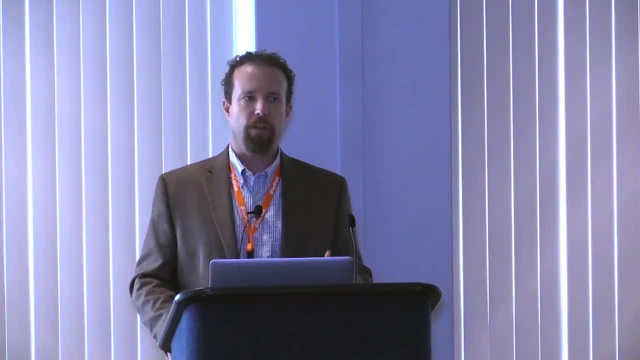 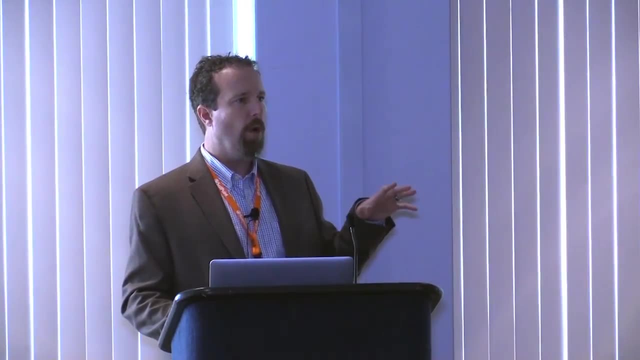 How difficult is it to put into production, maintain the care and feeding that must go into a security resource like this. So a lot of decisions have to go into what type of WAF you want to put in place, whether it's on-prem or in the cloud- very personal decisions for your. 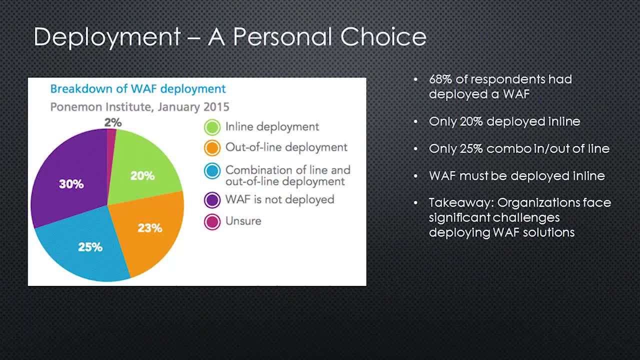 organization and what your security needs are. So the Ponemon Institute did a great survey where they asked a lot of organizations: do you have a WAF and if so, is it deployed in line or out of line? And 68 percent said we've got a WAF. 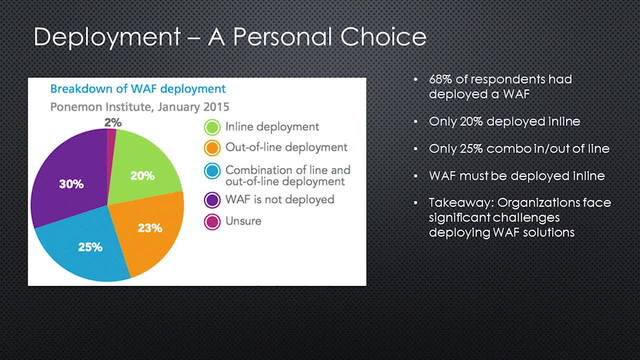 That's good- two thirds- But only 20 percent were deployed in line. So even with an in-line, out-of-line combo, that's still discouraging numbers when you have a security tool like that, but you're keeping it just on the sidelines. 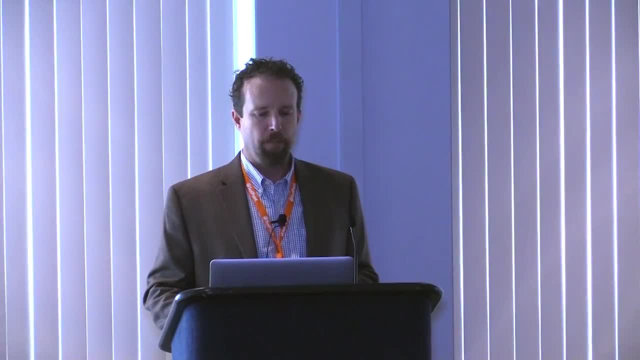 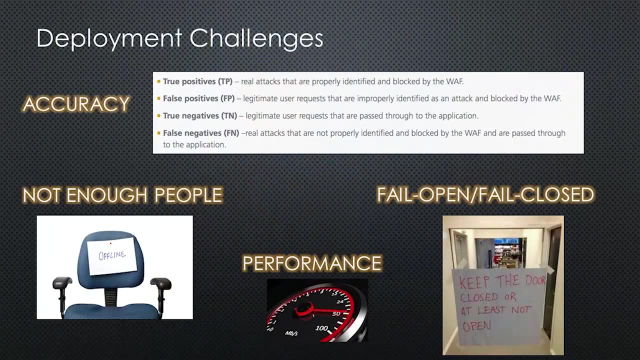 to let you know that you're being attacked. So the takeaway here is: organizations face significant challenge in implementing this type of security. What are some of those challenges? Gaging that accuracy, having an understanding of how effective is this, And you have to take into account the true 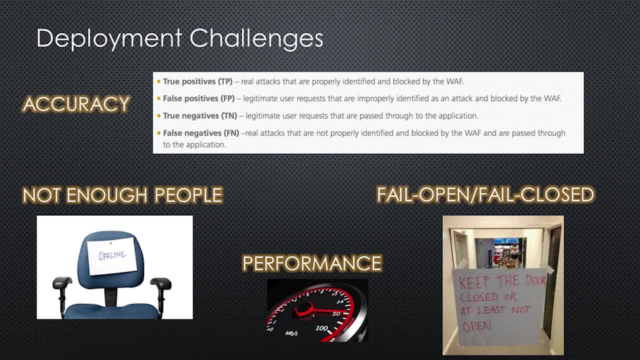 and false positives, the true and false negatives, and run those numbers to really come up with a true perspective of accuracy. And to do that, by the way, you have to have a test data set with known good and bad requests. You have to have something to test against and see how accurate your configuration was. 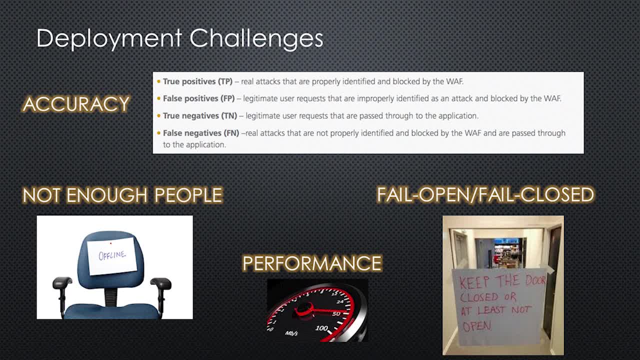 Not enough people, because it's not an easy task to do this effectively. That, one kind of speaks for itself. Performance might be forgotten from the security minded, but the other side of the house is going to yell when your security controls dramatically impact the performance of their web applications. 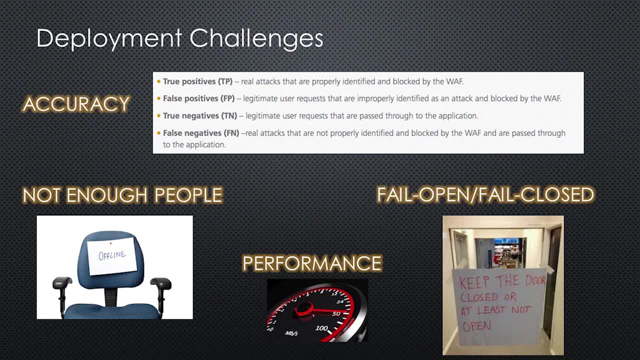 And finally the old fail open, fail close problem. Many traditional hardware WAFs load will fail open or fail closed, And so with fail open, they allow all traffic through, and fail closed, They let nothing through, And you have to choose between the lesser of two evils. 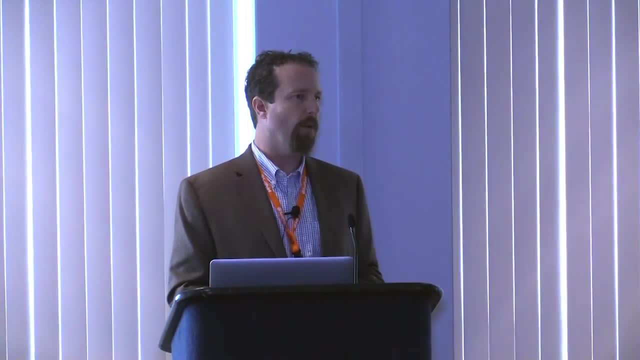 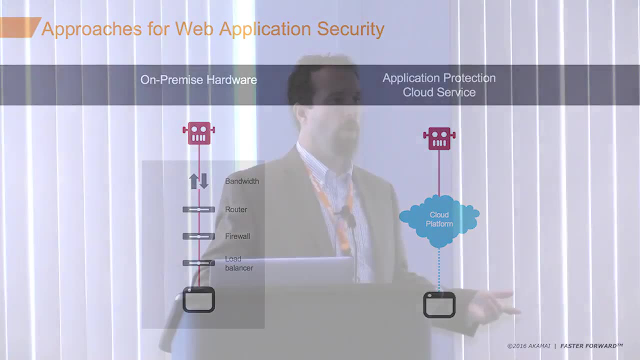 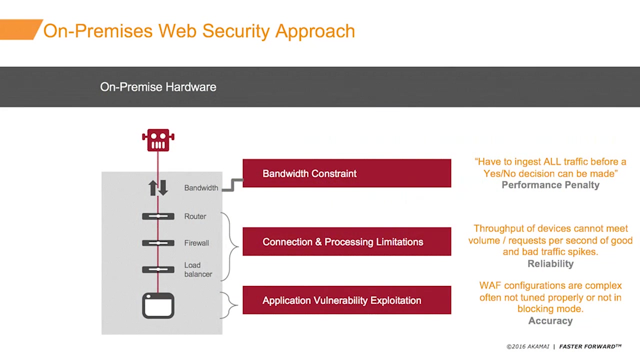 But both is evil. At the end of the day, you're impacting everyone. So there are different approaches, as I mentioned on prem in the cloud. which way you choose to go- or maybe both- depends on your organization's security needs and your resources on premise. 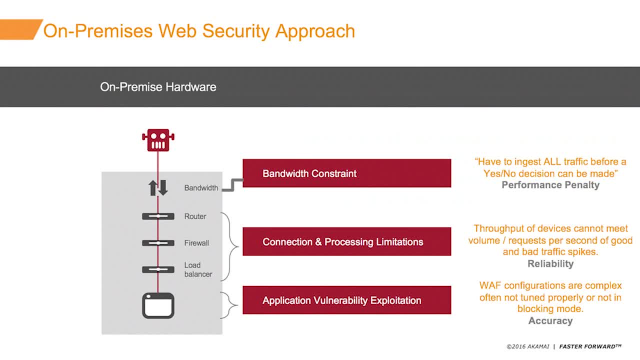 It's going to require more resources. But going beyond that, you have to actually receive that malicious traffic all the way at the edge of your network or right inside your network, So there could be constraints on bandwidth, performance issues, reliability- You can't have just one. 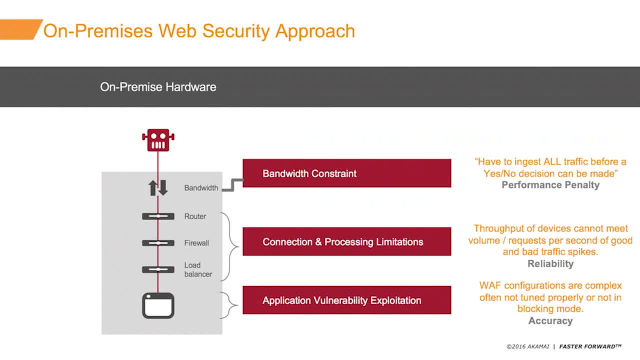 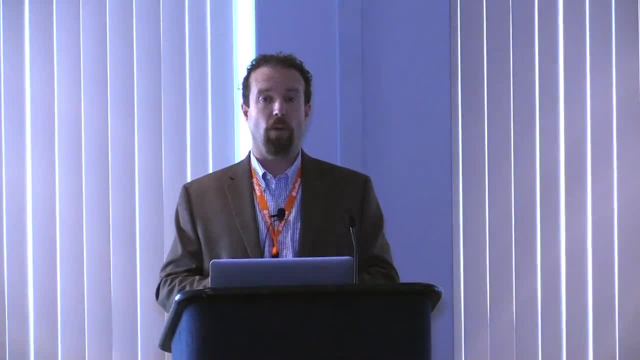 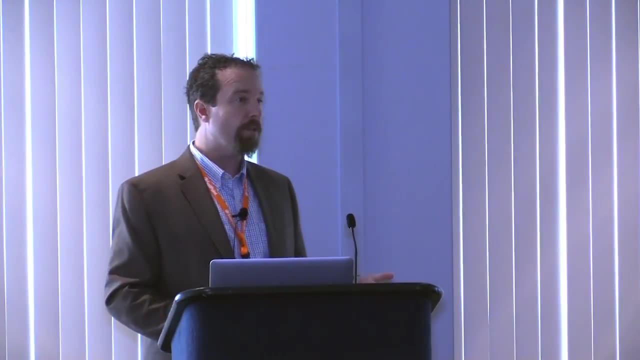 You have to have two maintenance contracts: FTE and the accuracy That all comes down to how well it's maintained. An accurate configuration relies on constant adjustments, tracking with the development of the application. The background in the cloud is another set of concerns. 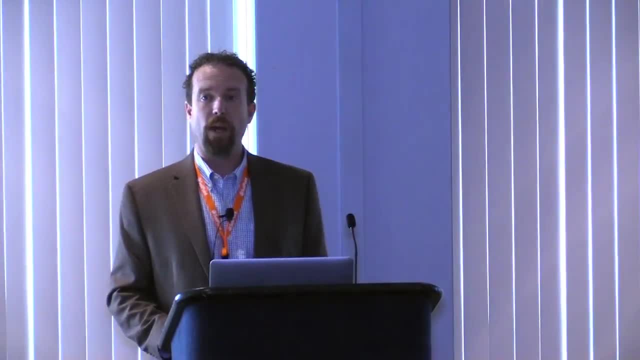 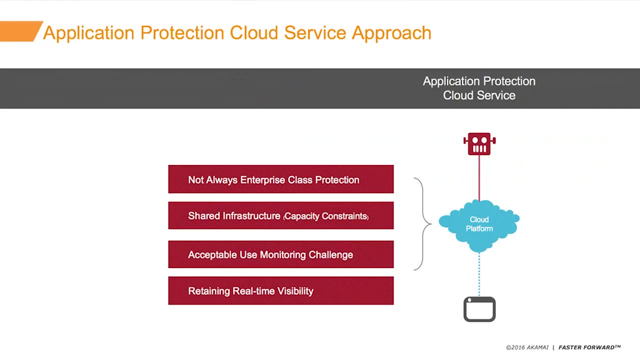 There's a lot of options And, like anything else you evaluate, they're not all the same, They're not all equal. So if you need an enterprise class WAF, you need to examine it from that perspective and make sure that's what you're getting with the features. 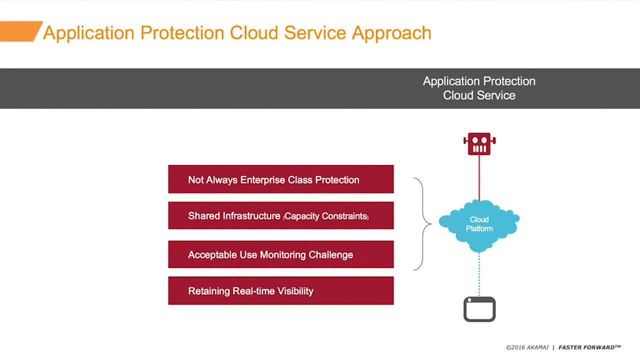 and functionality that you're looking for. Shared infrastructure: How big is that infrastructure? Does it have the capacity you need? Are you going to have to deal with acceptable use issues on a shared platform And then finally, retaining the real time visibility that you get with an on prem? 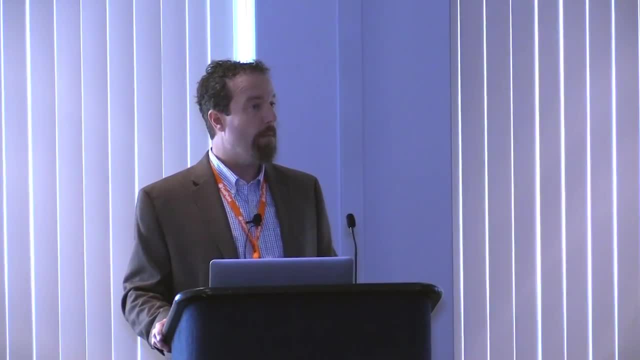 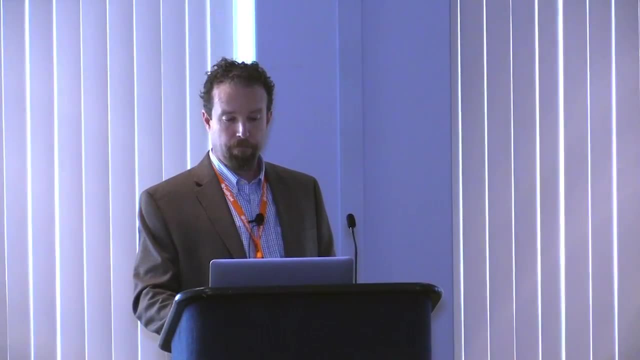 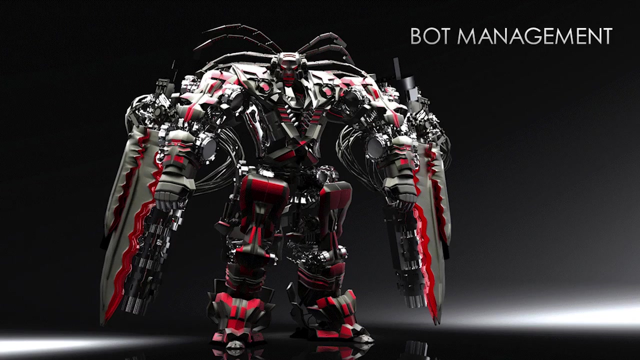 log an on prem, WAF and the logging systems that come with that. Being in the cloud presents its whole new set of challenges for getting that data in and then performing analysis. All right, let's go ahead and move over to the bot management problem. 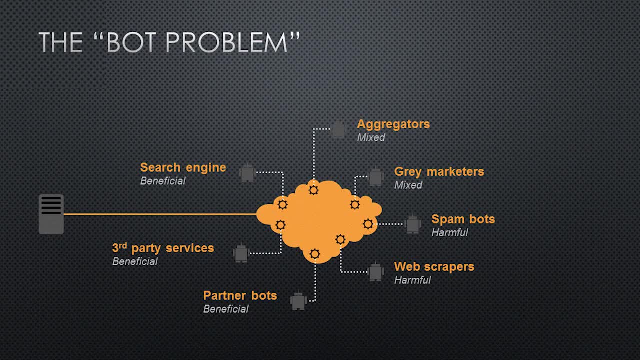 So, as I touched on before, there are a lot of different types of bots. There's good bots, there's obviously bad bots, and then there's a lot of bots in between, Where, again, we have that personal choice. But the reality is, dealing with bots is not like dealing with application attacks. 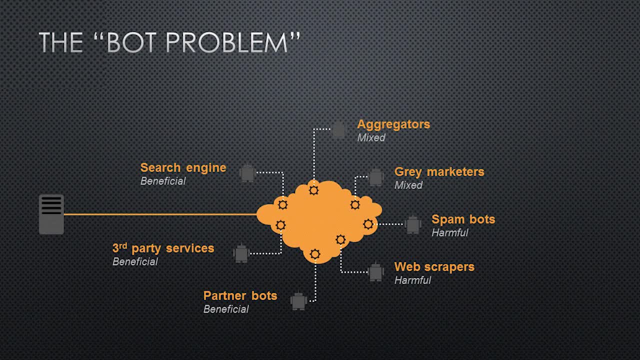 It's not black or white. where you see a malicious payload, We're going to stop that. We're going to send a 403.. We're going to deny it hard with bots. that has the opposite effect. So what we definitely need is a methodology. 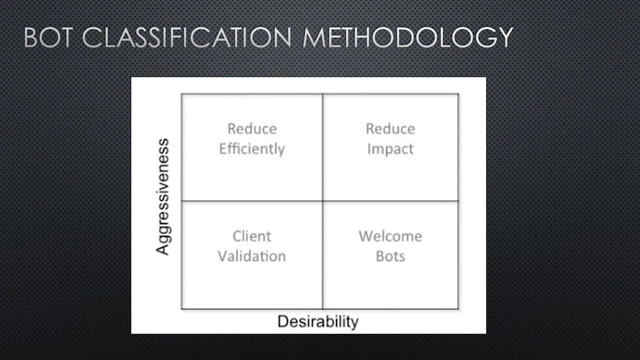 We've got good bots, We've got bad bots, We've got the ugly gray bots in the middle. We need a way to sort those out. So if we compare desirability on the bottom and aggressiveness on the top, in the bottom right, 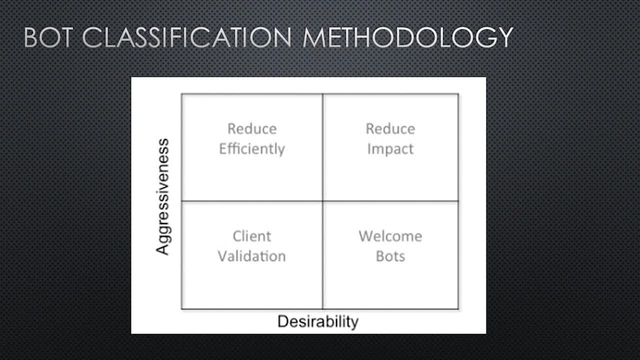 we see highly desirable, low aggressive bots. These are welcome bots, good friendly bots, things like search engines and SEO bots. In the top left quadrant we've got the opposite: Highly aggressive, not desirable. Think scrapers for fraudulent purposes. 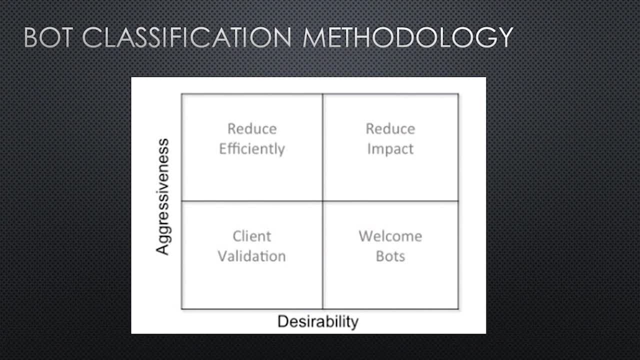 They're hitting you hard, They want the data and they want it now. These are pretty easy. The gray areas, the other two corners of this, the top right: highly desirable but highly aggressive. These could be other scrapers, These could be partner bots. 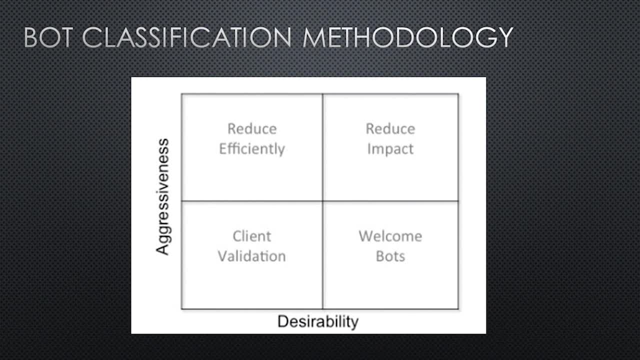 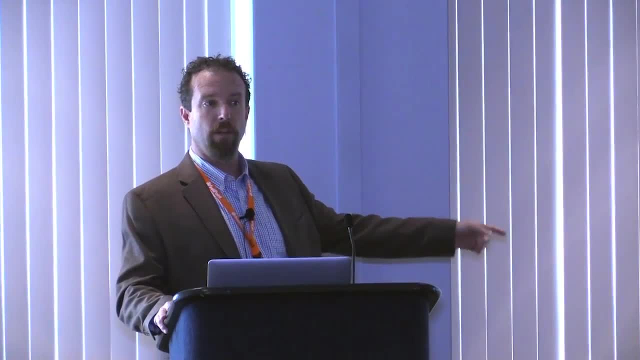 They don't really play along with the rules as the way you define them. Can you manage them in a way so that they still do what they need to do but not impact your resources? And in the bottom left low desirable low aggressiveness? 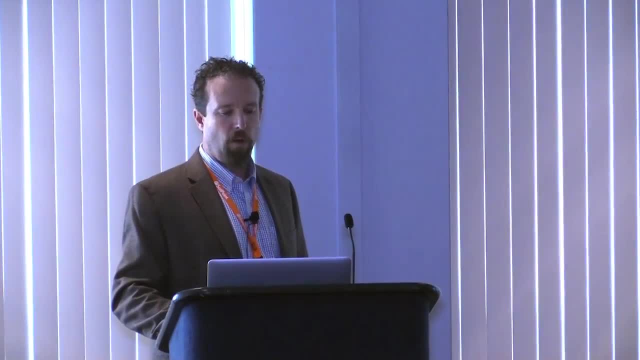 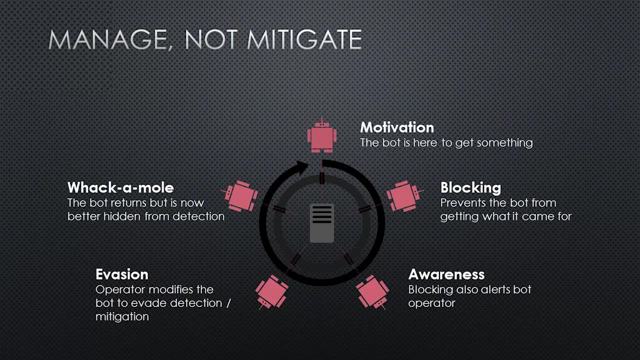 We're back to account checkers. OK, they're coming in low and slow and they're up to no good. So I mentioned that managing bots is completely different from managing application vulnerabilities in that it's not black and white. The motivation is there by the bot operator. 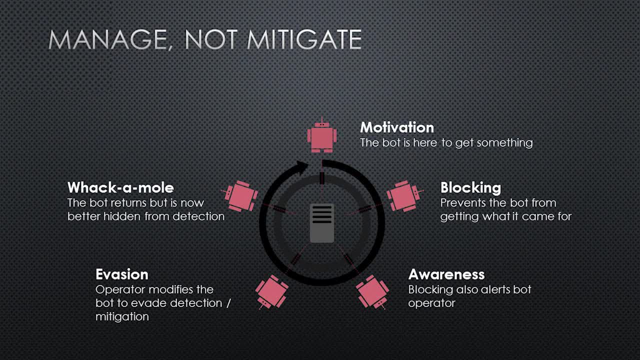 They're there for a reason. If you identify them in a way that blocks them, you have momentary success because you have now signaled to the bot operator that they need to evolve and morph their bots and their processes so that they can continue to get the information they need. they want. 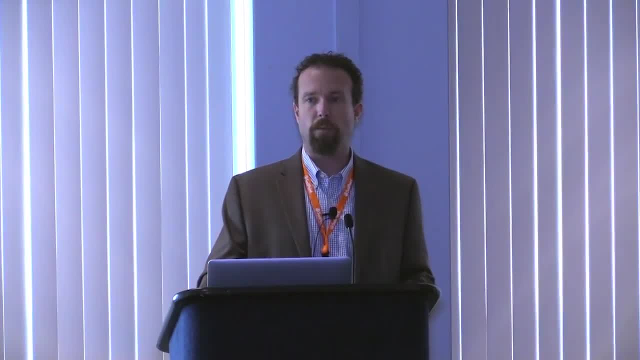 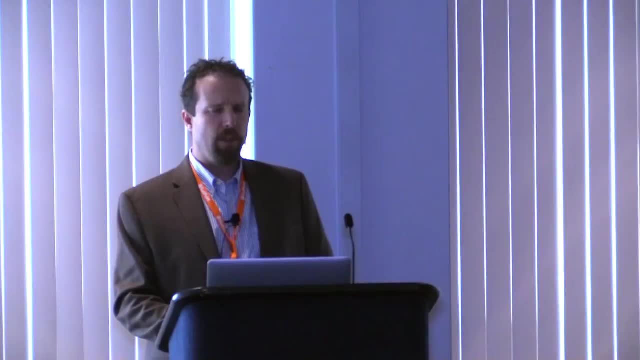 And so you're in this vicious circle of whack-a-mole, where you're chasing, playing cat and mouse and they're getting harder, faster, stronger to detect. So, instead of the bot management solution, what if you could do things that would allow you to detect the bots and manage? 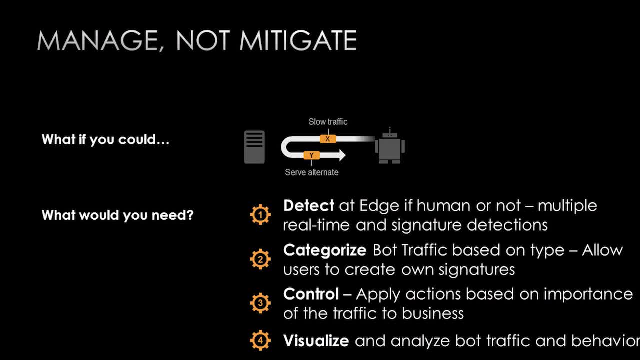 them in a very granular fashion, maybe slow them down, serve them alternate content, not necessarily alert them. what would you need with a flexible fabric like this? Number one, you have to first determine: is this a bot or is this a human? 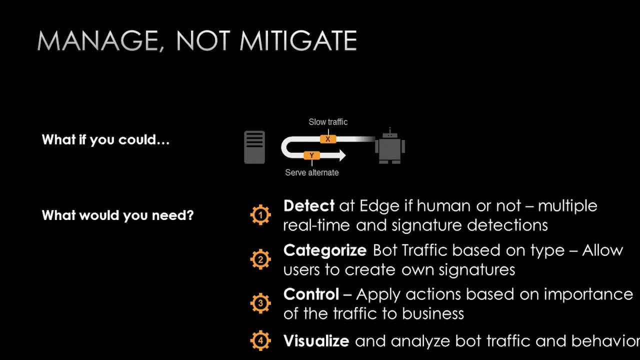 Seems simple, right, But you need multiple signatures and real time detection techniques to be able to dig into that. for the more nefarious bots, OK, because they will evolve and signatures won't work. after we identify human versus bot, We have to categorize them. 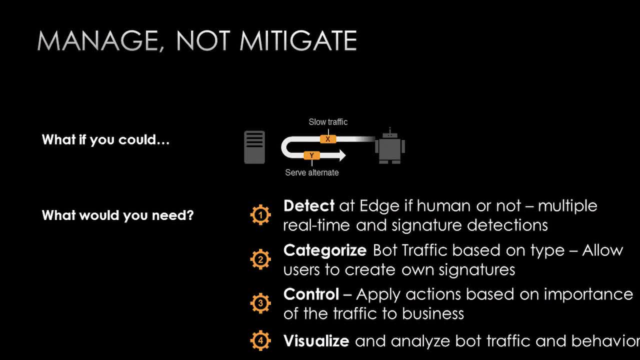 And having that level of granularity then affords you to say: this bot is in this category. Therefore, when we go on and apply controls, we can apply the controls in just a granular fashion, Having a wide tool set of how you're going to respond to the different categories. 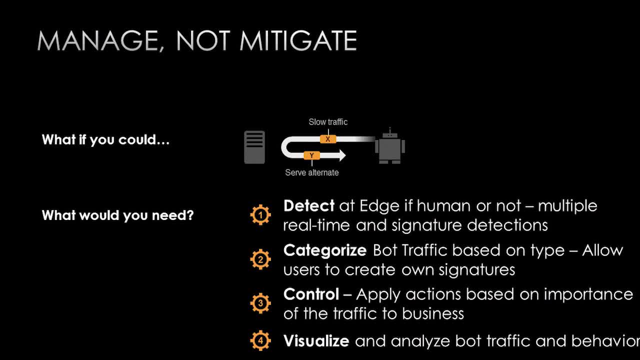 increases the chances you're going to be effective. And finally, visibility. like all security controls, We need to have the ability to get those logs, need to have the ability to perform analysis on the data we're generating to make sure we're effective. 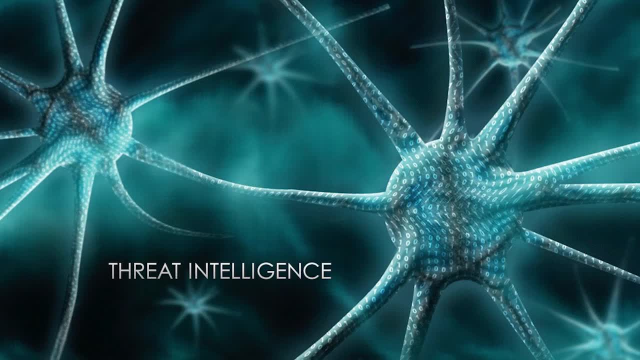 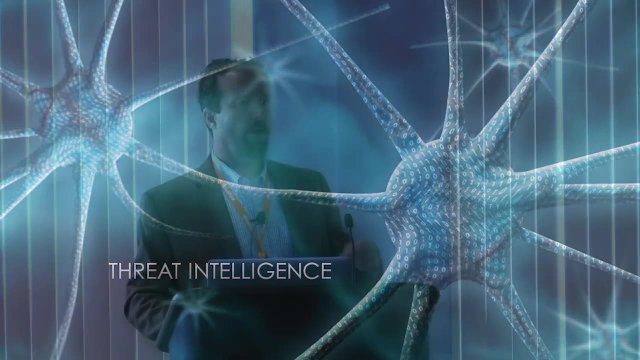 And last but not least, the third pillar, threat intelligence. So I hope that some of the previous things I've mentioned you can see from this frame of perspective that having solid threat intelligence enhances the capabilities of web application firewalls. it enhances the capabilities of a bot management solution. 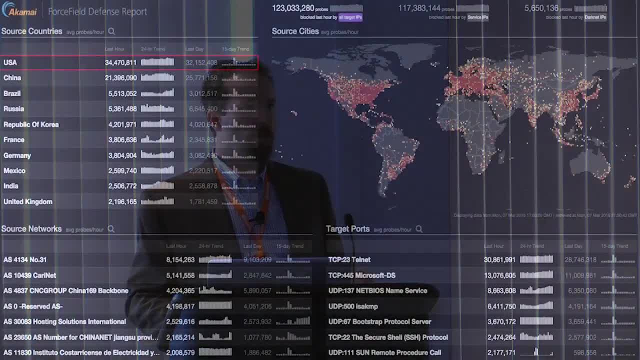 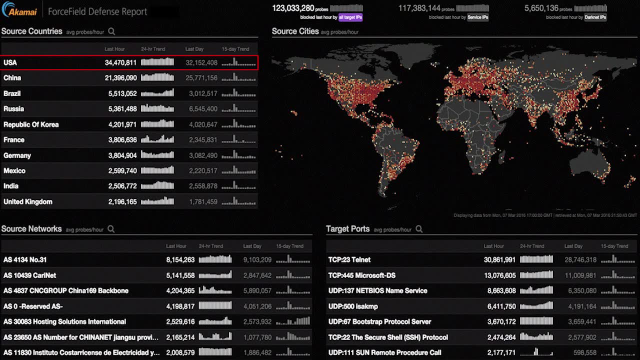 So what types of threat intelligence are we talking about? Third party feeds, you can have them from multiple vendors. This is an example of some threat intelligence we generate. Remember the scanning, probing data I showed earlier in the presentation? This is where we're gathering that and correlating that. 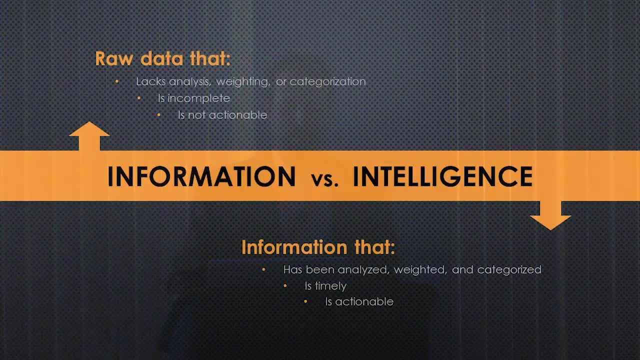 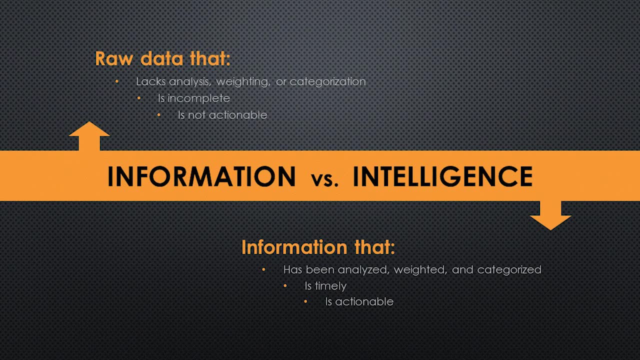 Have to point out US again, top source Got to secure our stuff. So what is intelligence? What is threat intelligence? Information versus intelligence? Well, information is really just the raw data. It's not been analyzed, It's not been weighted. 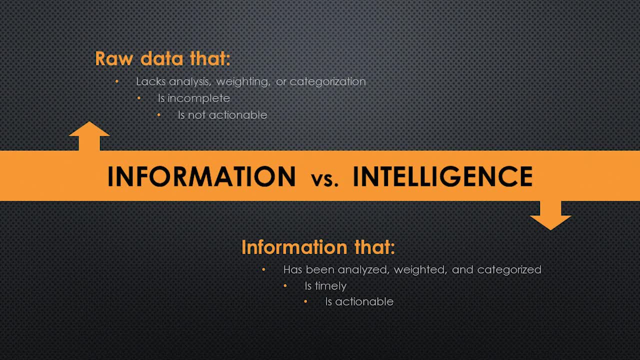 It's not been categorized, There's no correlation across the data, It's really not complete in any way and it's not actionable. Raw data is just that. It's of no good in a security implementation. But intelligence is when we've applied analysis. 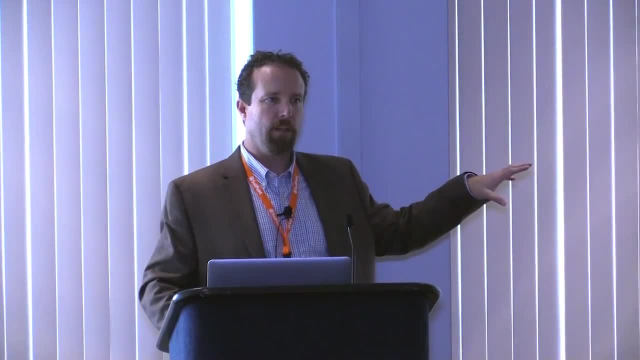 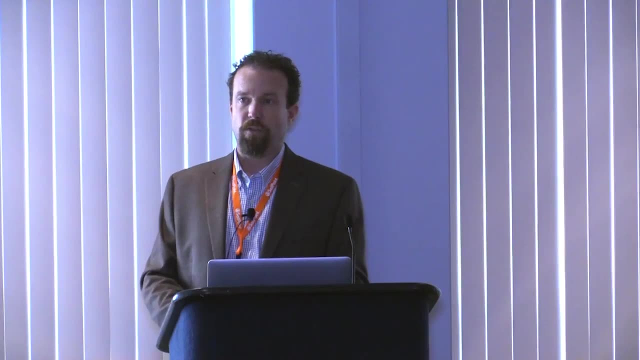 We've applied weighting and categorization to that data, We've correlated it and then we've made it available in a timely fashion so that you can take action on it. That's at a high level. the definition of intelligence, threat intelligence data. 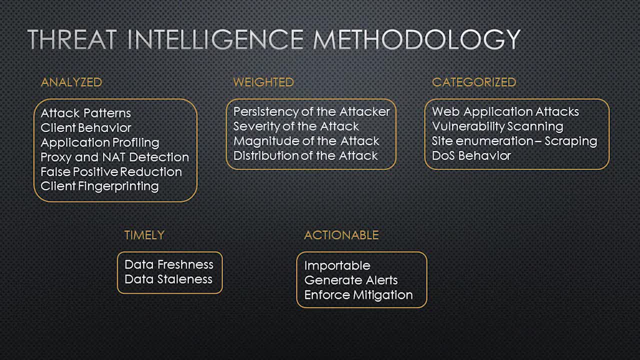 But from a methodology perspective, I think there's five things that are important. We need to evaluate the threat. intelligence feeds we're looking at from these perspectives. How is it analyzed? How are heuristics used to identify attack patterns? looking for common attack behaviors? 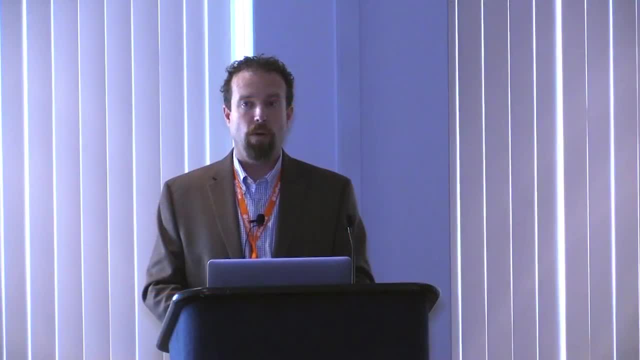 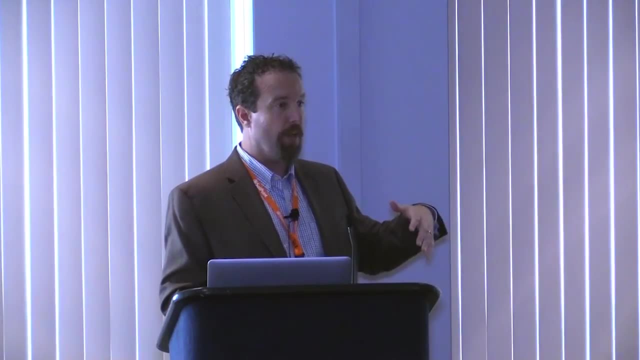 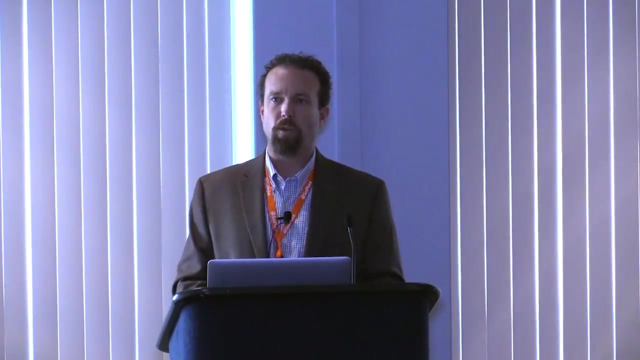 What heuristics are used to evaluate the client behavior against legitimate users. Heuristics for application profiling, so that we have an understanding of the underlying infrastructure, to give us context. Heuristics for proxy and NAT detection to rule out source IPs that may appear. 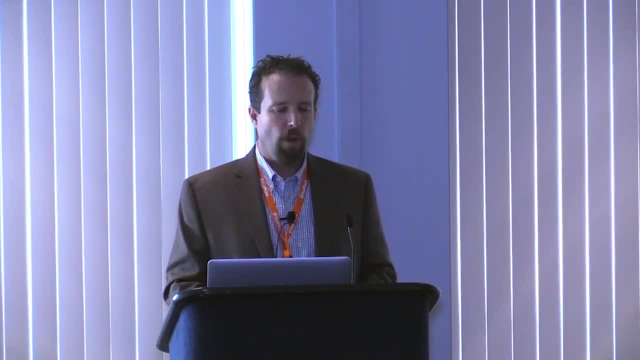 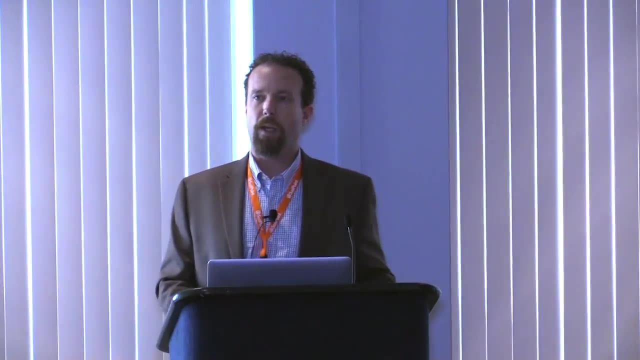 malicious because there's one bad apple in the bunch. Finally, client fingerprinting. Oh, false positive reduction. I skipped that one. You've got to have heuristics that go through there and look for FP. You've got to perform multiple layers of that. 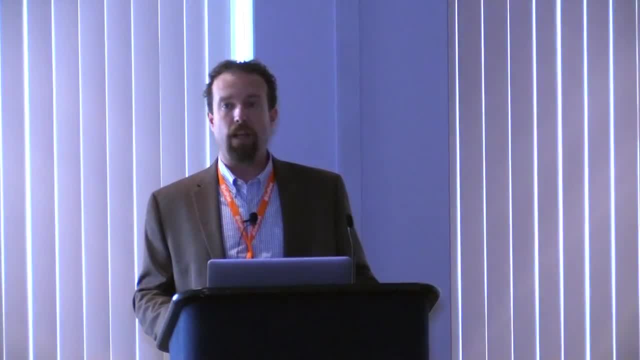 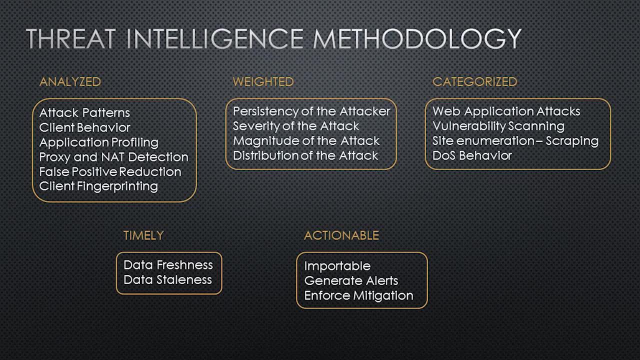 You have to vet this data, and then client fingerprinting, taking it to the next level, beyond the IP, and actually fingerprinting the original client itself. Number two in this methodology is weighting the data. Okay, Looking at four things: the length of time the attack occurred. 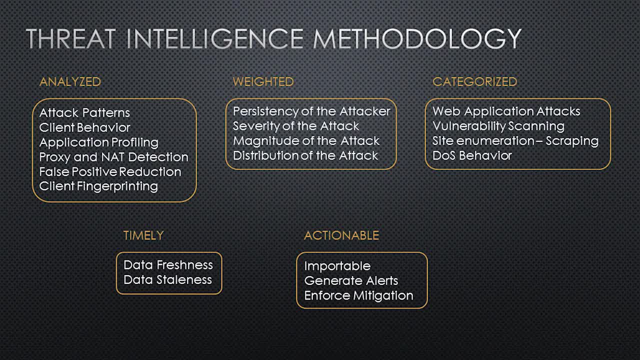 the persistency of it, the potential impact of the malicious payloads, the severity, the magnitude of the attack, the number of attacks that you witnessed from this particular source- whether it's a client or a source IP- and, finally, the distribution, the number of hosts that were targeted. All of these things can be used to factor. 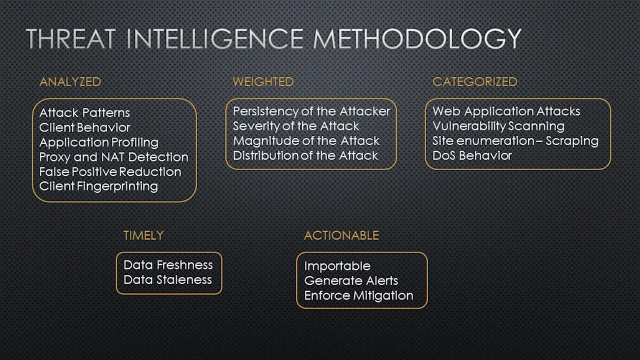 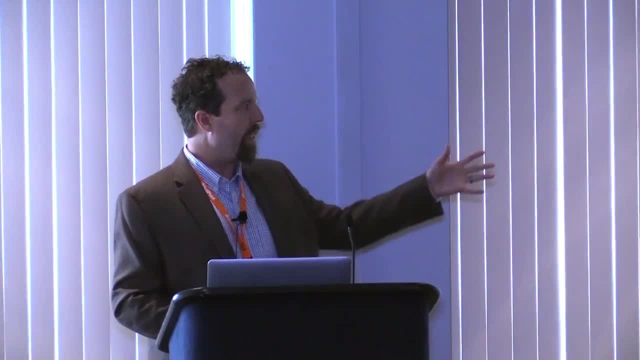 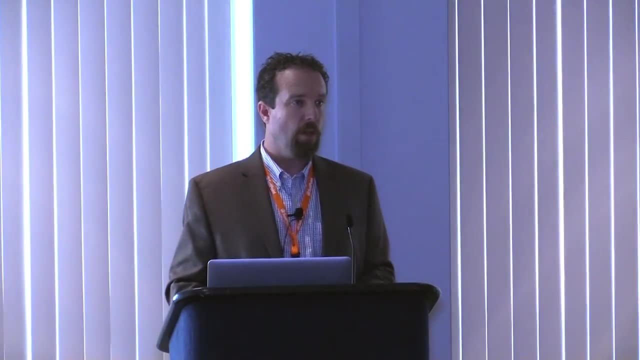 in the weight of the score within the threat intel feed. Number three: categorization. I really love categorization, but if we're categorizing it, we can break it down into things like web application attacks, vulnerability scanning, site enumeration and availability attacks. 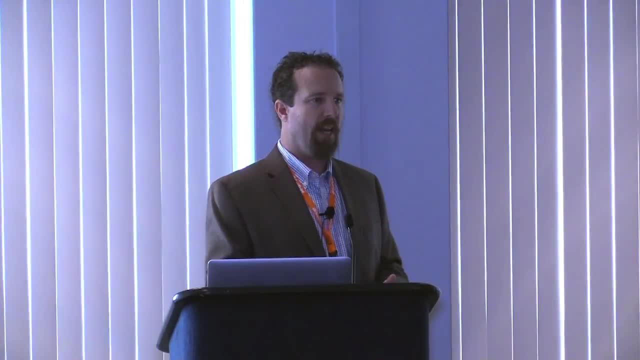 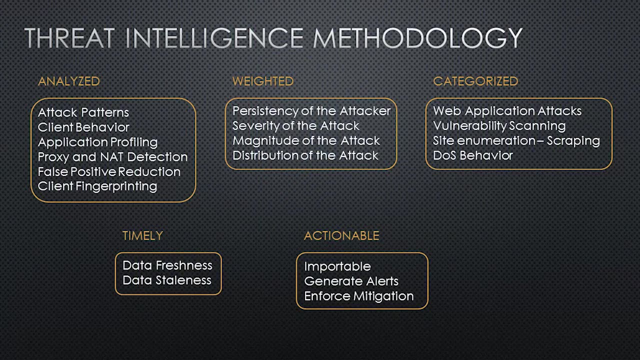 So if you have a category, a weighted score and vetted analyzed data, you're well on your way. but we still need number four. That data has to have freshness and staleness. You need to have perspective First. you need to get the data quickly. 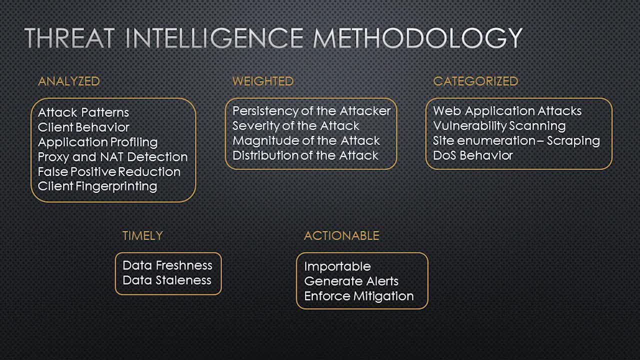 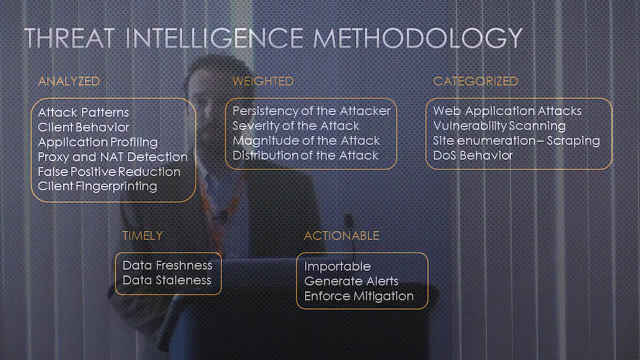 and then you need to have perspective over time on how old that data is. You have to decay those scores and there has to be a consistent applied manner to that. Finally, of course, it has to be actionable. So you have to have the means to incorporate that data to generate alerts. 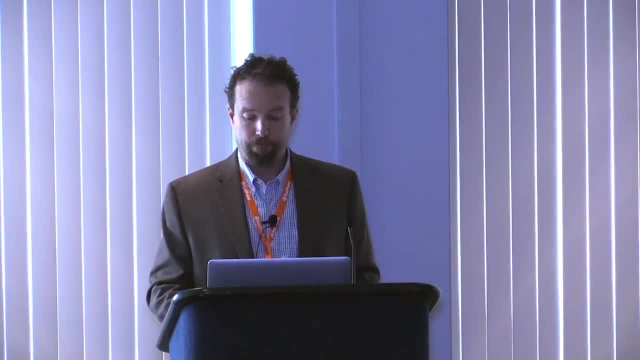 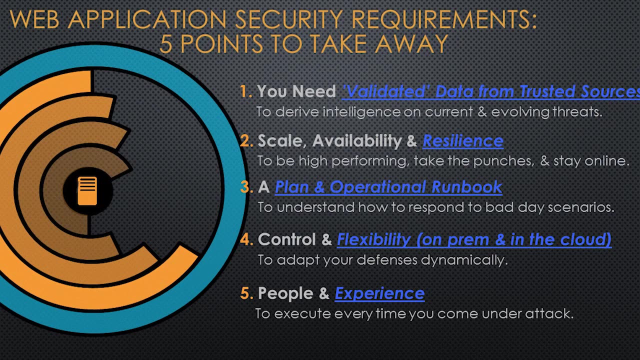 and enforce mitigation and utilize denies. So I want to kind of wrap up with five points. I like to give five takeaways whenever I have a discussion. Number one: so these are web application security requirements. Number one: you need validated data from trusted sources. 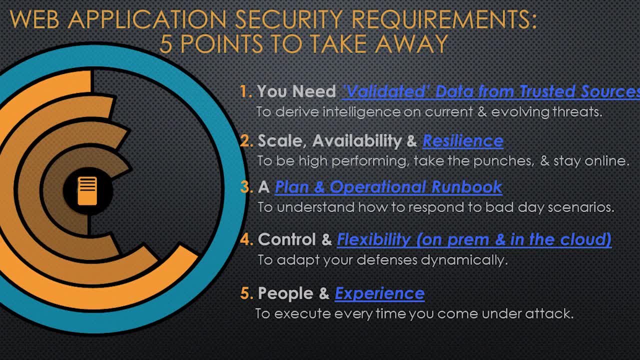 Just because it's a client Intel feed doesn't mean it's been vetted in the same way that you would vet it. so you need to take the steps and go through that exercise. Number two scale availability and resilience to be high performing. 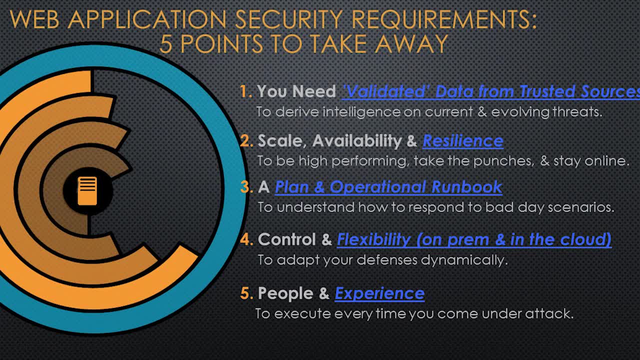 stay online, withstand the attacks and continue to perform at scale. A plan and an operational runbook are critical when you're having a very bad day. Number four: control and flexibility of your resources, whether they're on-prem or in the cloud. 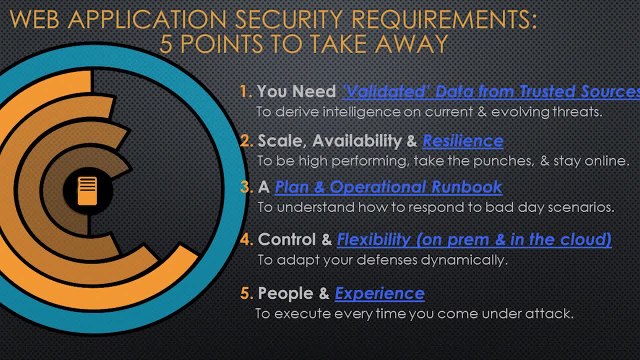 give you that flexibility to adapt to an attack when you're having a very bad day. And most importantly, I think, are the people and experience you have behind the controls that you put in place. Those people need to be able to execute and perform, no matter the circumstances.